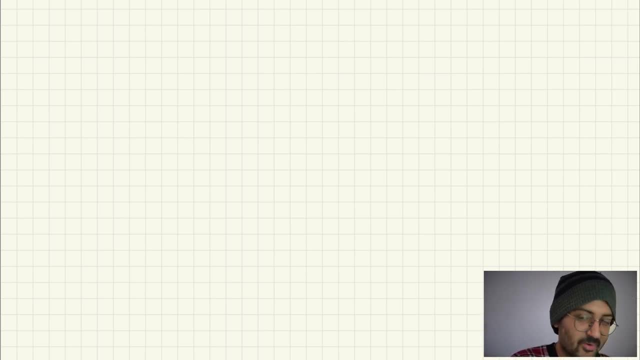 Huffman, decoding, whatever you want to call it, But we're going to learn about encoding, decoding. So you know, for example, you have zip files, you know you have compressed files, and then you use your unzip tools and software and it unzips the file into a nice little folder. 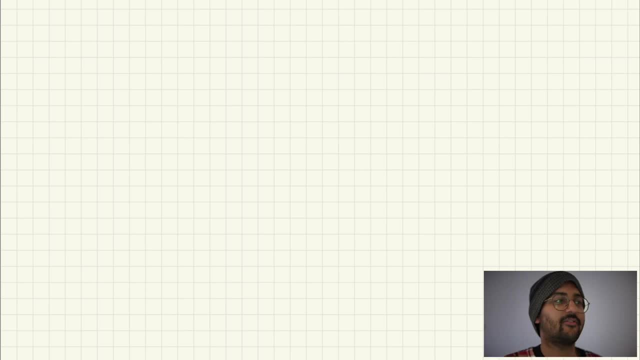 So the compression algorithms, you know, reducing the file size. how do we do that? What sort of algorithms do we use? A very popular algorithm for that is Huffman right, Huffman coding. So we're going to compress, we're going to learn how to compress. 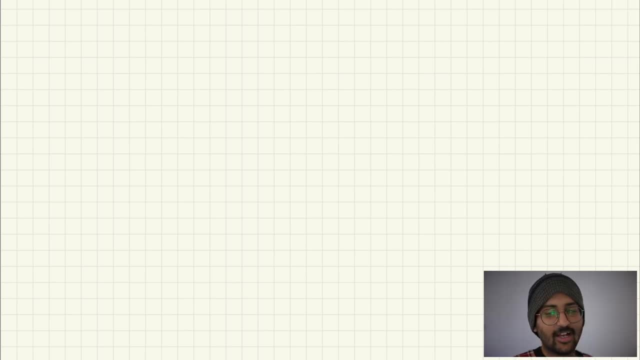 files in this video. So very exciting. right And Huffman coding has a lot of real world implementation implementations. it is used like in fax, when you used to send fax machines and like text things like that and your GZIP and your zip files and things like that. Many codecs like your songs, like mp3 of 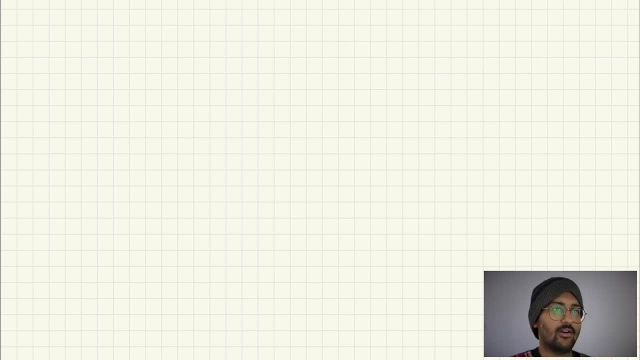 your photos like jpg and all sorts of things, Right? So let's learn about Huffman encoding. how does Huffman encoding work And how are we going to reduce this size? one thing you have to understand is any information, any digital information in this world. 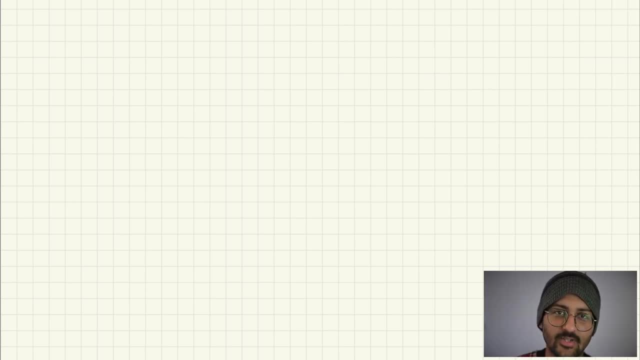 anything, it's in the form of bits of ones and zeros. any 4k, 8k video, you have, any picture, you have anything you have, it is all in the form of zeros and ones. so that is how we know that we can compress here anything. right, but how do we actually compress? what do we do? so, first thing, 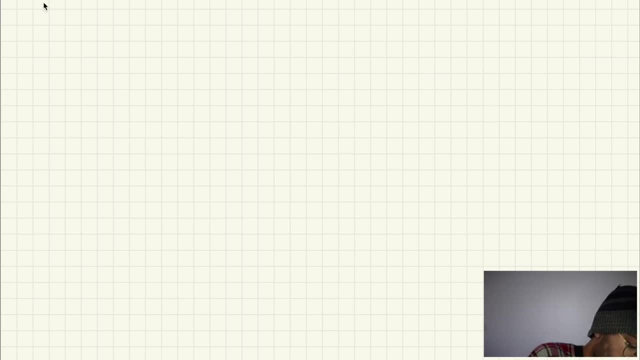 i want to share is that huffman coding? if you talk about huffman coding, this is a lossless algorithm, so data will not be lost. okay, lossless data compression. lossless data compression- all right. sometimes, when you're video calling with people or you're uploading videos on youtube and stuff, some frames may drop. 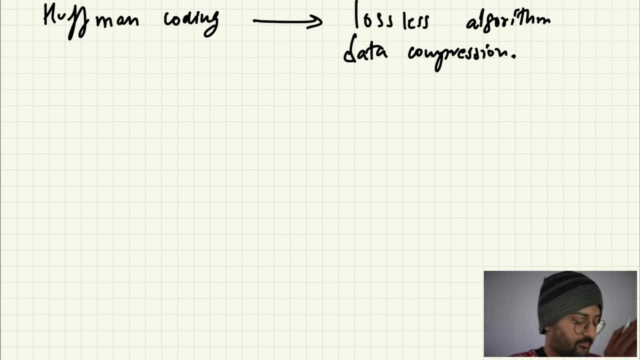 okay, so that's not lossless. some data is lost, so where do we get started with huffman coding? okay, so let's say everything in ones and zeros. so in this example, let's say: i take a string. okay, i'll take a string in java. i can say: let's say i have a string. 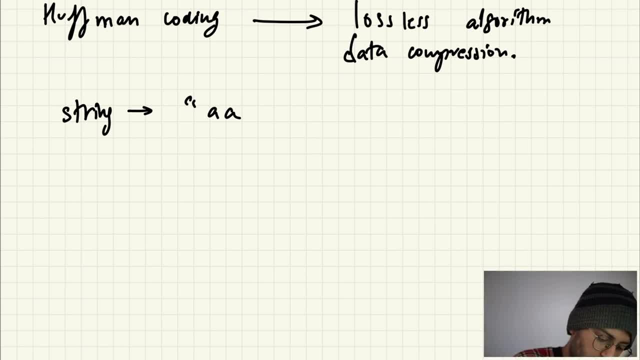 that is something like a, a, b, c, d, a, g or whatever. this is a string. what is the space taken by the string in java? what is the size of one character in java? two bytes. so this is equal to total. how much spaces is taking two bytes or? 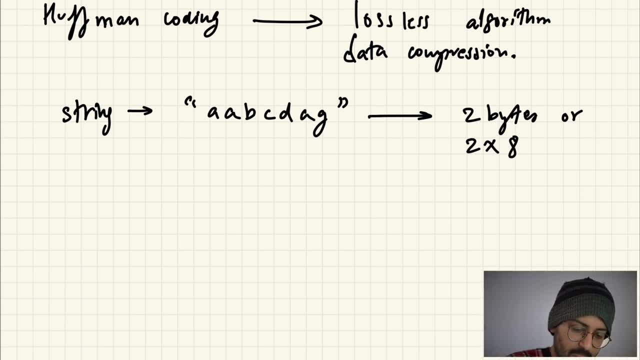 two into eight. two bytes per character, so total characters: how much do we have? seven, so seven into two characters, so seven characters. each character is two bytes, so 16 bytes in total. okay, and how many bits in total multiplied by eight? so 112 bits. okay, 112 bits. 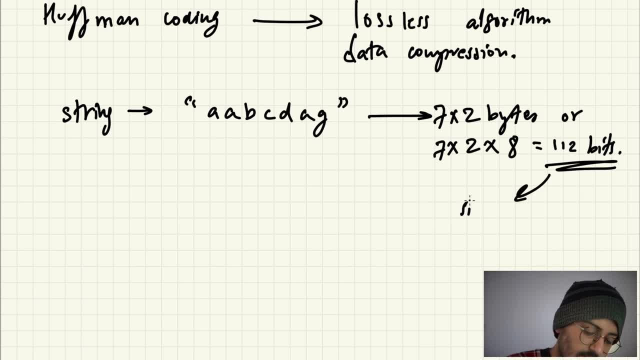 it is taking. so this is the size of your file, for example, or your data. what does compression mean? compared data compression mean I want to store the same amount, but in less number of size, less number of bits. are you able to understand? that's what compression is. you have a. you have a. 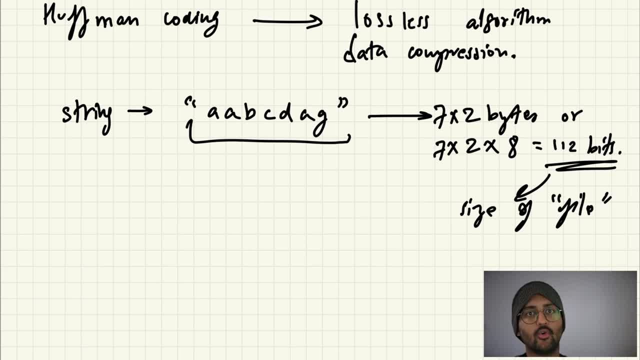 picture that is like 10, 10 MB. you compress it down to 2 MB or something, sometimes right. so data should not be lost. string should be as it is, but I have to reduce the number of bits it takes to store it. how can we do that? so? 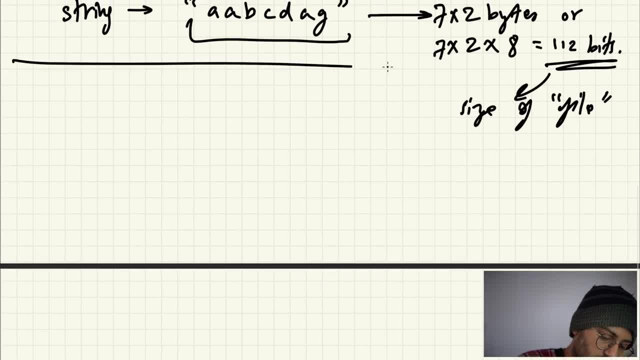 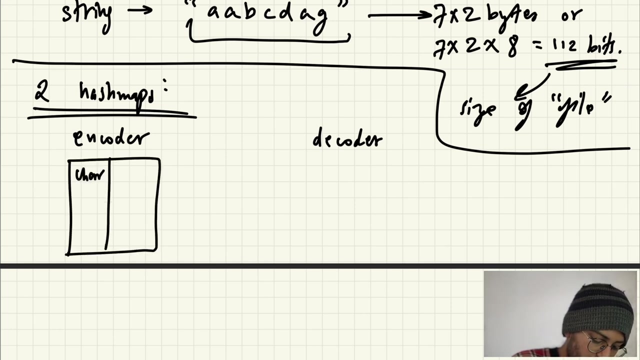 for this we use Huffman coding. let's see what Huffman coding is, how it works. so we will take two hash maps. this is now we're talking about the Huffman coding algorithm. okay, so we will have two hash maps. we will have an encoder and decoder. this will have key as character and string. here I will tell you what it is in, just 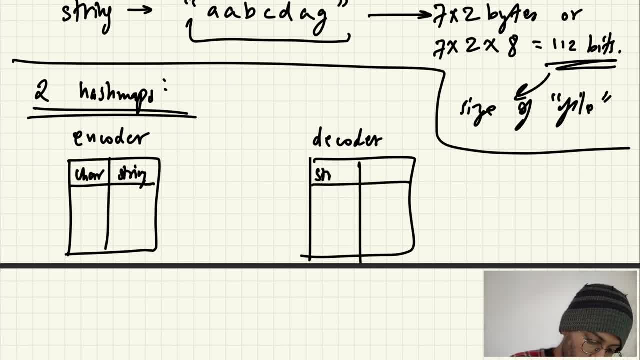 a minute. string here char. here a b c d, a b c d. so encoder and decoder. encoding means that you transform a sequence of like some character, into bytes or bits or whatever you wanna call it. decoder is you take that sequence of bytes and convert that into character. 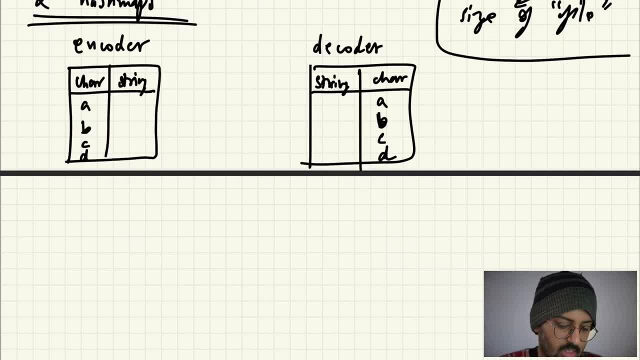 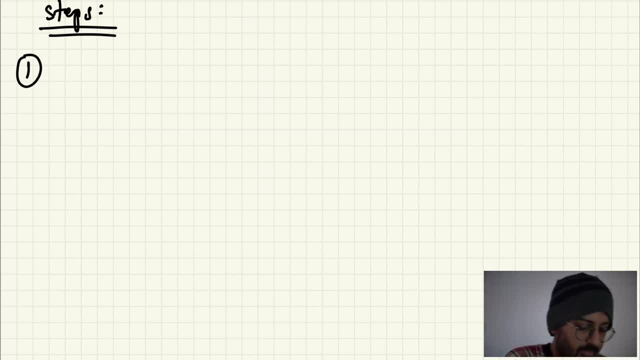 you'll see in just a minute. so what are the steps? so the steps are very simple for Huffman encoding. Step number one is we are going to actually get like a pattern. you know, for every character in the string, For example, we will pass the string. that is point number one. pass the main string. 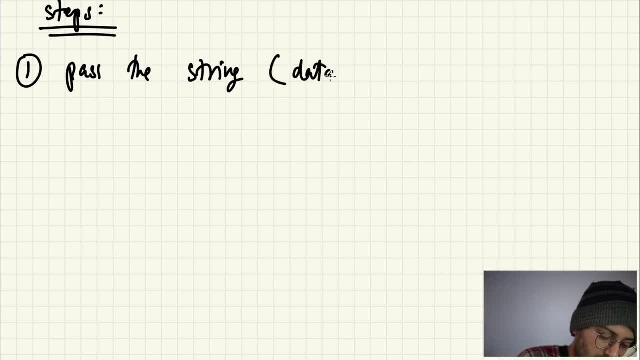 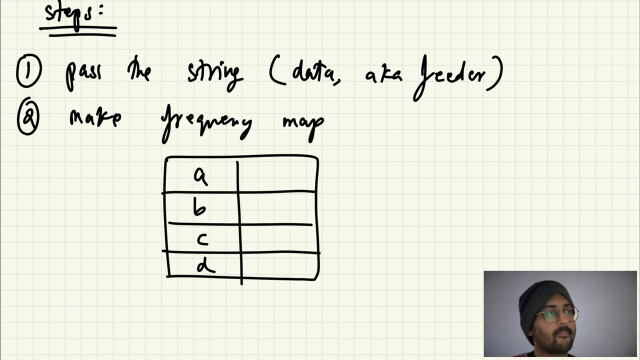 that you want to compress. This is known as your data, also known as pdr, and we are going to make a frequency map of it. Make- we did this in the last section- count sort frequency map. For example: A, B, C, D. A is coming sixty times B is coming thirty times C is coming. 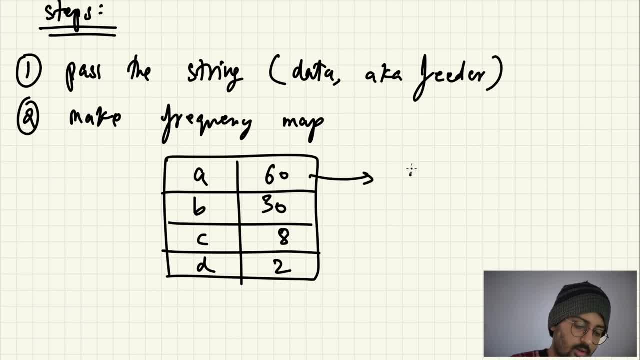 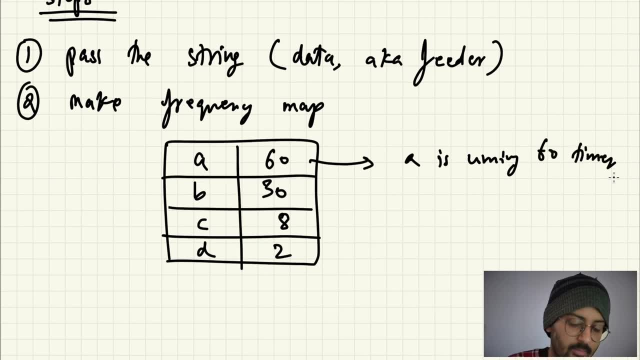 eight times. D is coming two times, okay, A is coming sixty times in the string that we whole message that I want to compress. So actually in this video we are actually making a program where you will be, you know. 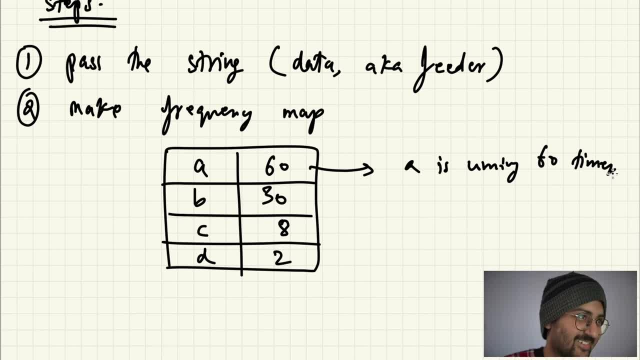 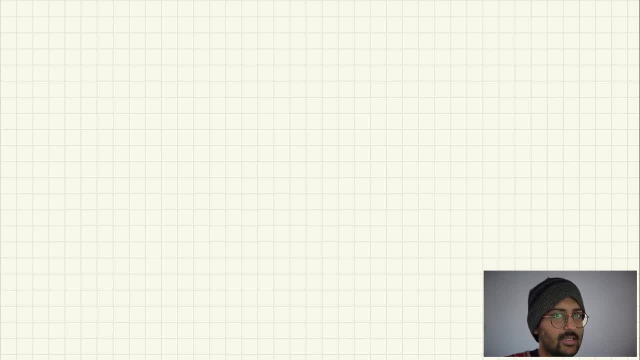 able to send decoded messages to your friend. so pretty cool, okay? So frequency map is made over here. Now what I am going to do is step number three for every key in the frequency map. for every key in frequency. Okay. 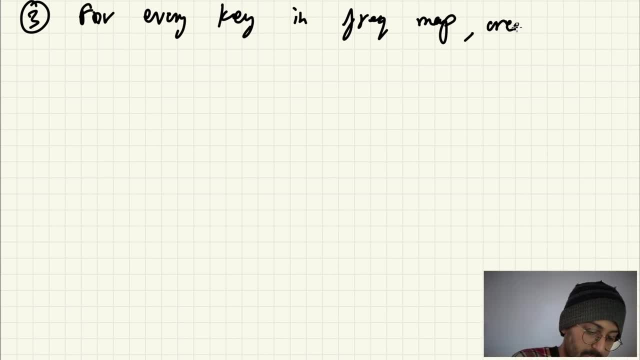 For every key in the frequency map. I am going to create a node. create a node and insert that node in a min heap. We have done heaps before. this is also known as priority queue. we have done this before in our previous lecture, right. 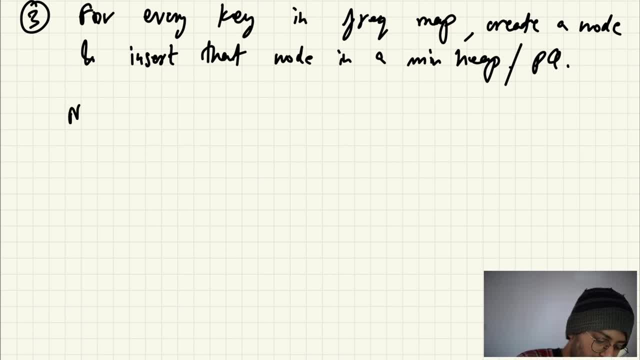 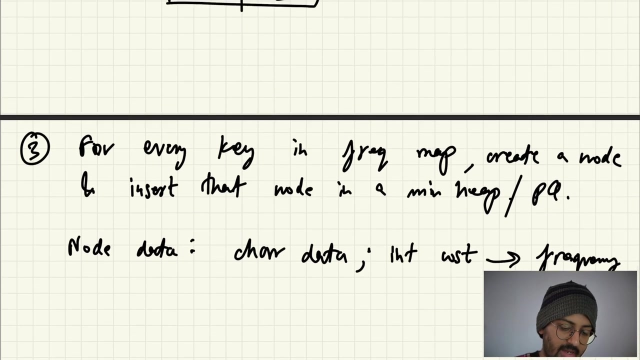 Kunal. what does this node look like? Node has this data. It has a character data. it has an int cost. okay, A cost is what Cost is the frequency? that's it okay. So for if data is equal to A, then cost is equal to number of times it is occurring. 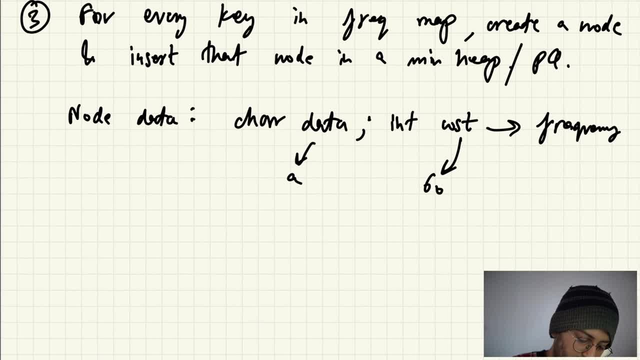 sixty. Okay, It will also have a node left. Okay, It will also have a node left. Okay, Left and right, Which is going to make a tree and using that tree will create our pattern And using that pattern, we will encode and decode our string. I will just show you in: 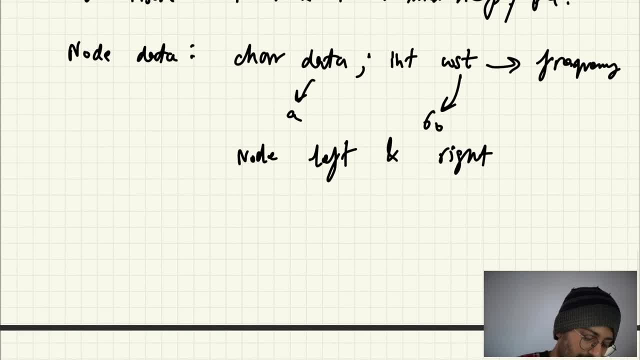 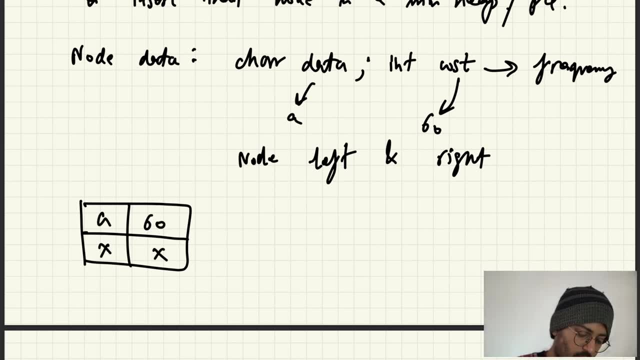 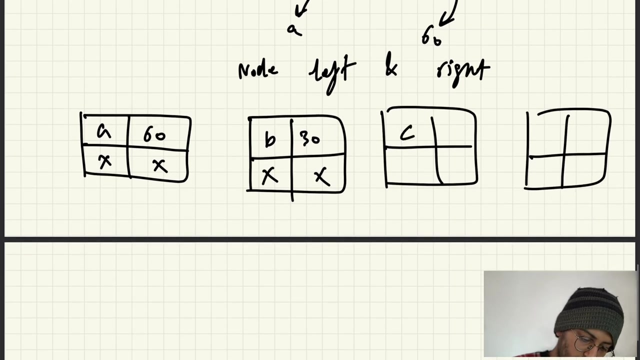 just a minute, Okay. So initial heap will look like something like this: Nothing in the left and right: A cost sixty, B thirty, Okay, Okay. C and D. Initially left and right, nothing. What is the C and D at eight and two? 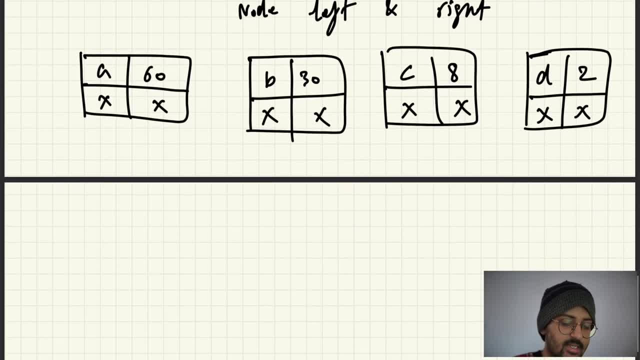 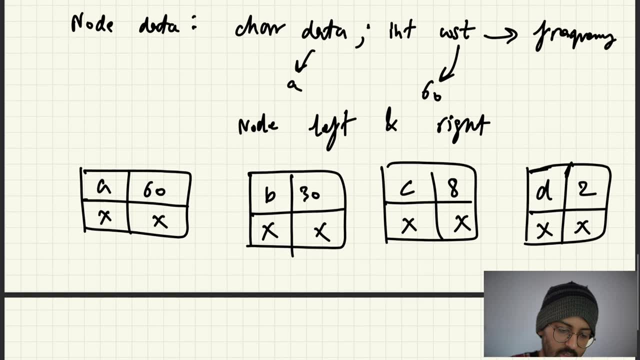 Eight and two. Okay, Since it is a min heap, which item will be removed first? The smallest one based on the, based on the, let's say, if it's min heap, based on the cost, D will be removed first because it is min heap. 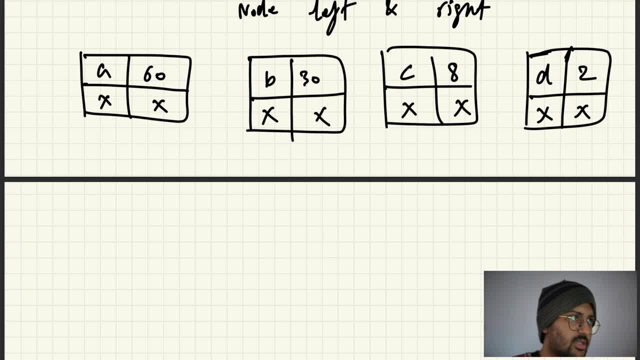 If you don't know heaps, watch the heap video. Okay, I'm showing you step by step. So next step, step number four, go through the heap. remove two elements from the heap and combine them. So remove two elements from heap and combine. 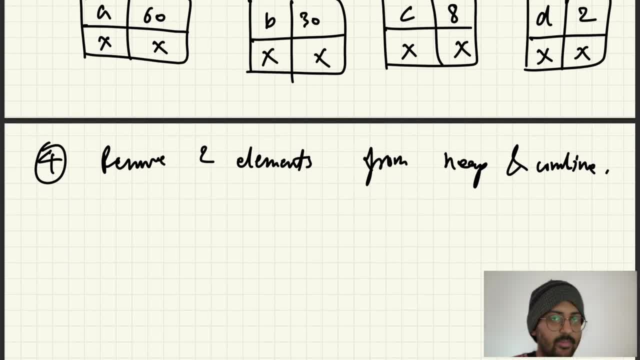 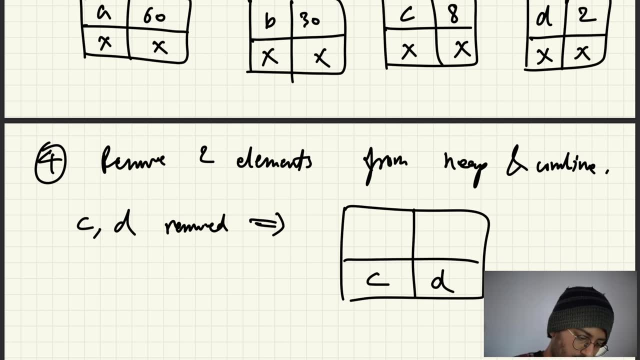 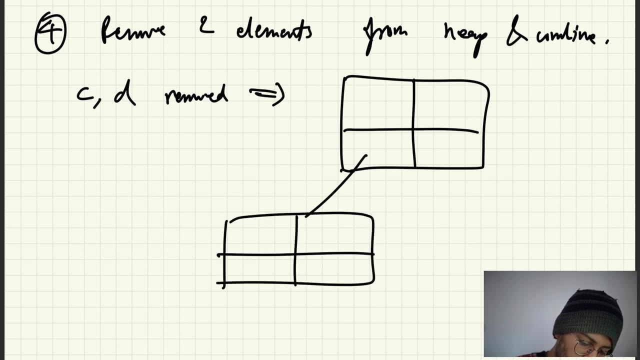 Which two will be removed. D will be removed, C will be removed. Okay, C and D removed, because it's min heap. So if I combine it, I will say C and D. I can just write like this: Node left is going to be equal to C, Node right is going to be equal to D. Cost of C. 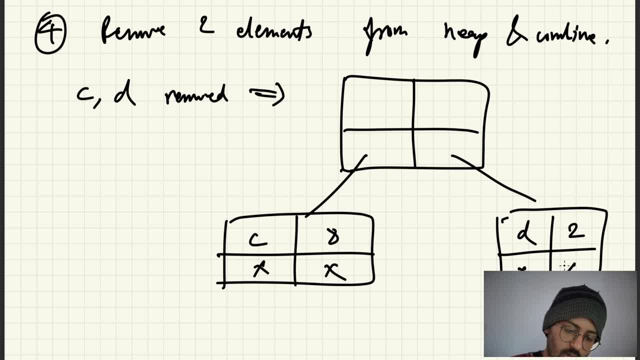 eight, X, X, D is two, Left, nothing, right, nothing. So you can see how I'm forming my tree. When I remove two nodes from the heap and I create another new node, the left of that node will be the one of the removed ones. 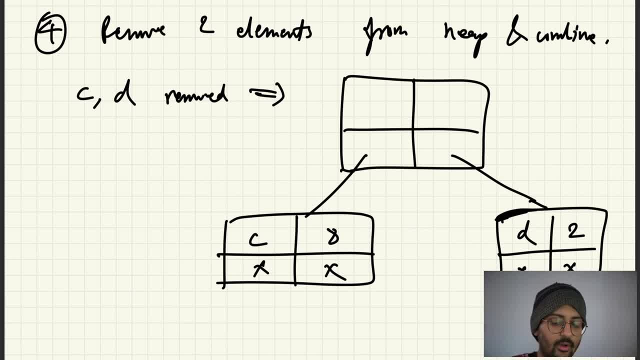 Right will be the another removed one. Now you'll be like Kunal. how do you know C is left and D is right? Can it not be D right, D left and C right? Yes, Doesn't matter, This can be interchanged also. 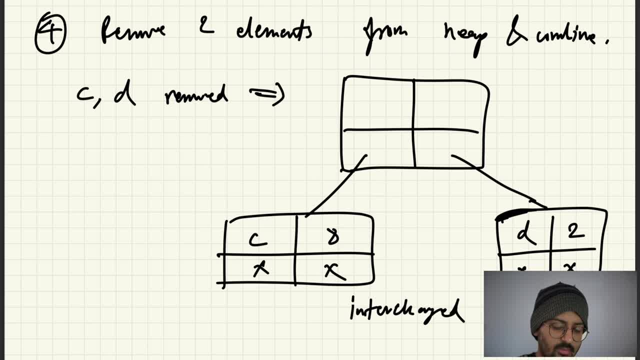 Interchanged. order does not matter, Okay, Okay. Order does not matter Of the left and right. Okay, Interchanged is phi, This new one. this will be null, no name. But what is the cost? now, eight plus two. 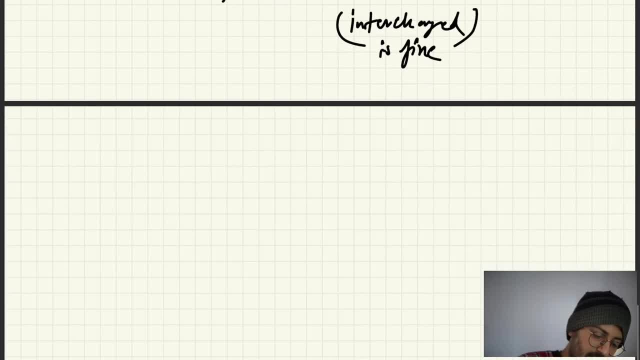 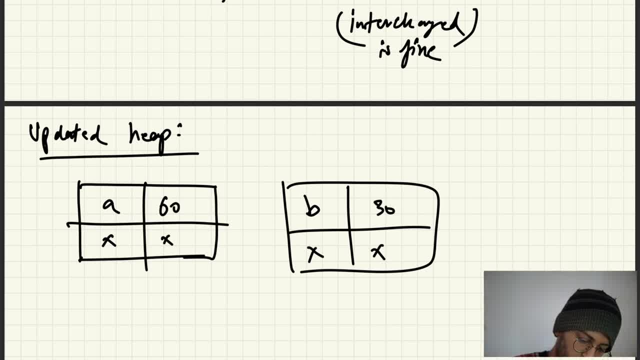 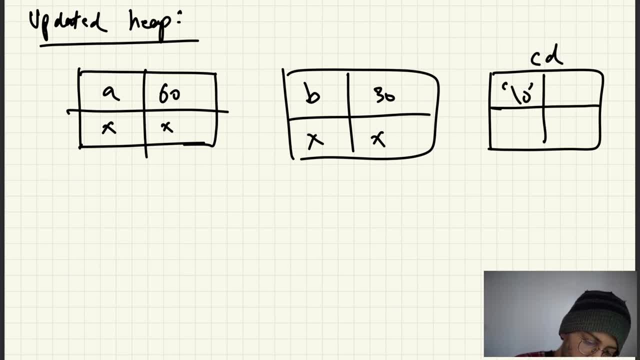 I have this one: C, D- This is null, no name as such. this value is ten. This is having C pointer and D pointer easy. this is what my heap looks like now. sound good. now what will be removed? we have three nodes now. this node, this node and this node mean heap will remove two. 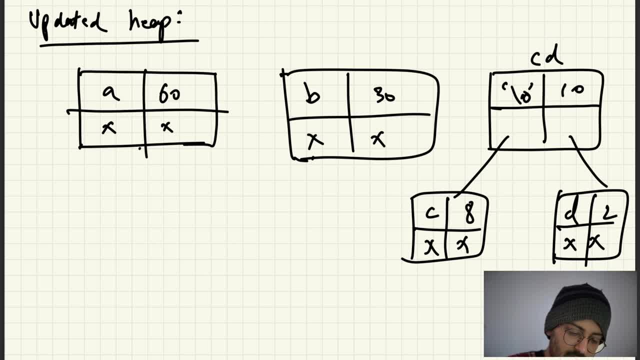 nodes. again, what are the two smallest nodes? don't consider the C and D. now, okay, it's because it's a part of these three nodes, like it's a part of this node right now. this one, it's a part of this node. so in total I have three nodes. only C and D are now. 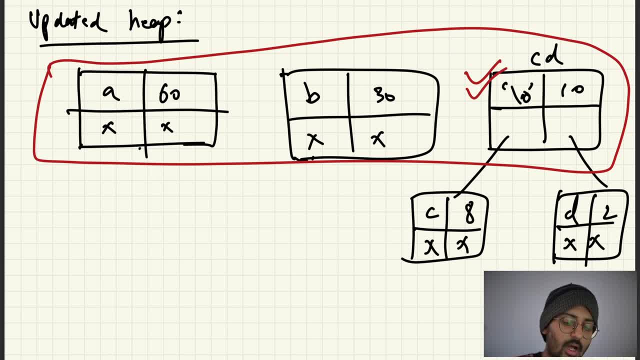 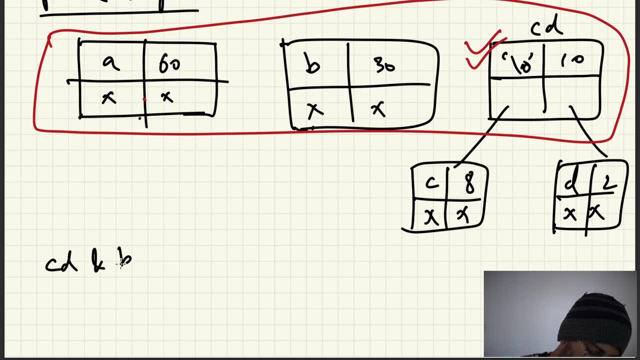 part of left and right child of this node. don't be like Kunal. now we have five nodes, no one node. one node, one node, okay. so updated heap will be what? what will be removed? now you tell me two smallest ones, 10 and 30. so C, D and B. 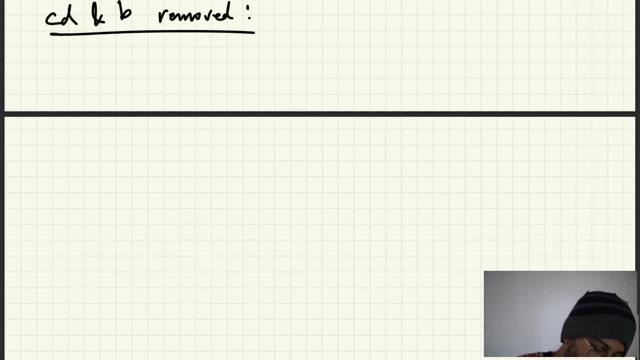 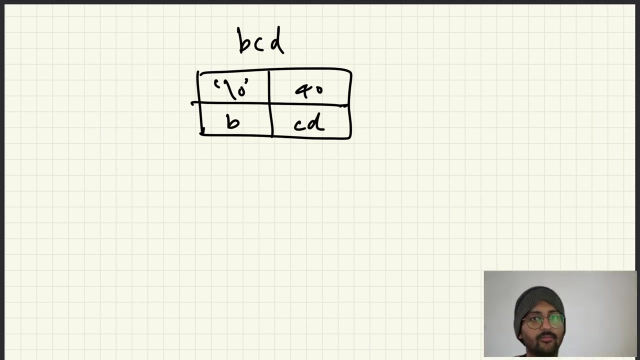 removed. so C, D and B will be removed. it will form B, C D. if it forms B, C D, right. so here I will have null 30 plus 10, 40. here it will have B node, here it will have C D node. okay, updated heap. 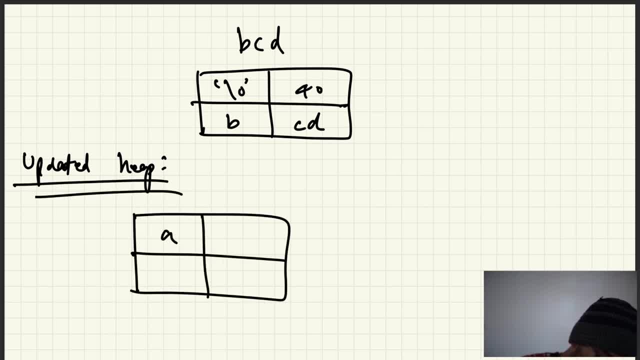 A, 60 and B, C, D. this null is just nothing. I'm not giving it any name as such. cost is 40 B and C D. only two nodes are left, so I will leave it as it is for now. so I will leave it as it is for now. so I will leave it as it is for now. so I will. 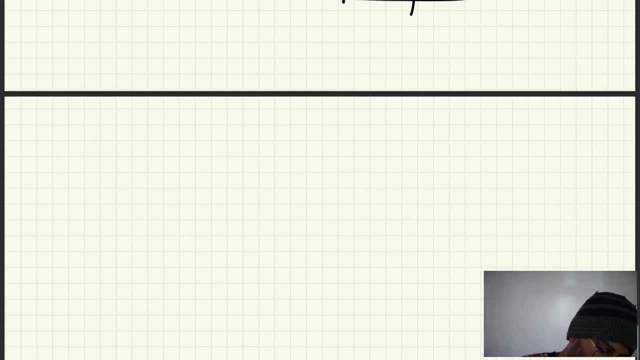 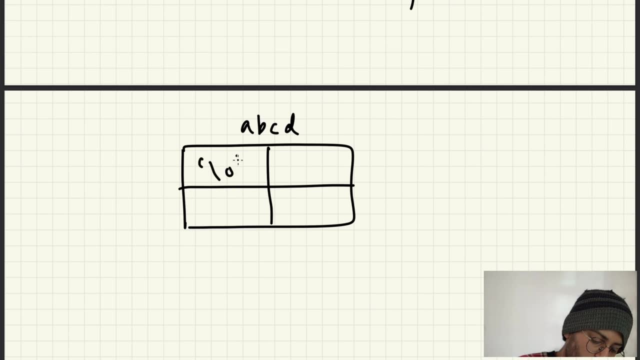 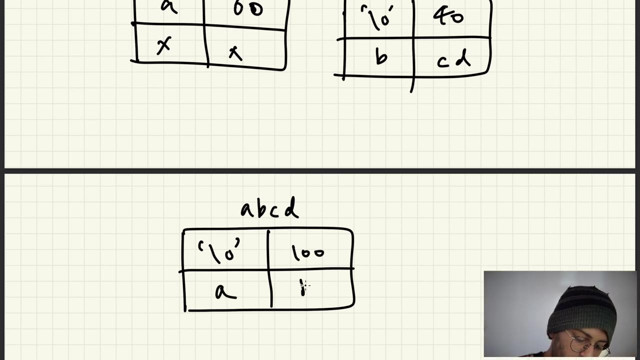 combine and remove these two nodes and combine those. so it will be formed A, B, C, D. right, this will be 60 plus 40 hundred. see the pattern, see what I'm doing: A will come here, B, C, D will come here. now, only this node is in the heap. 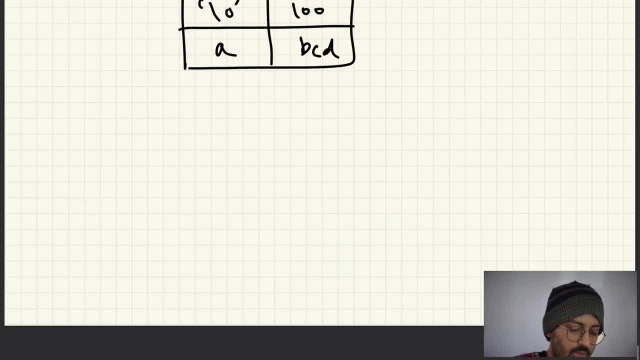 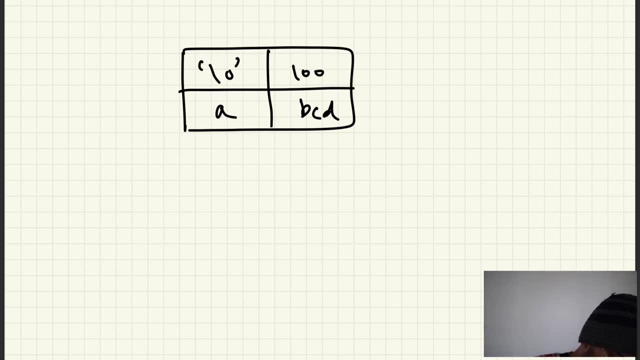 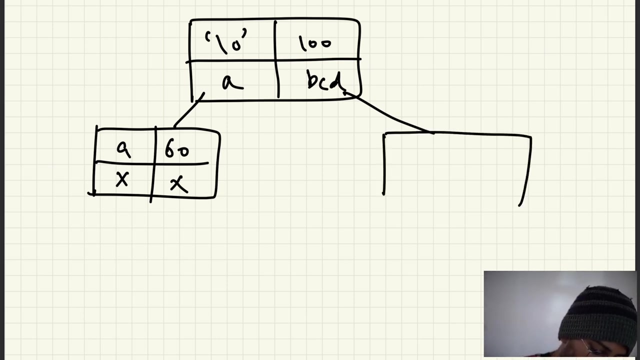 okay, so what does this node look like? what does this look like if I expand it? okay, if I expand it, what will it look like? A basically just means A over here now. B C D means what we know. we know what B C D means here: 40 B and C D. 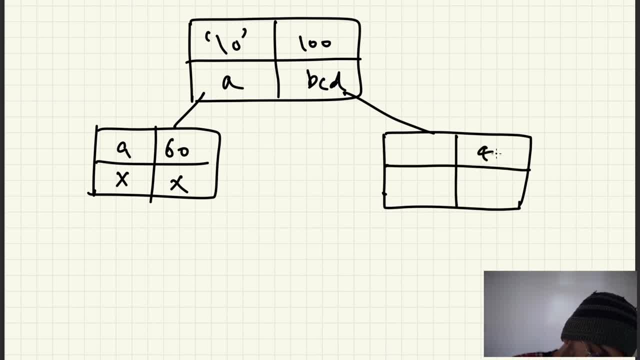 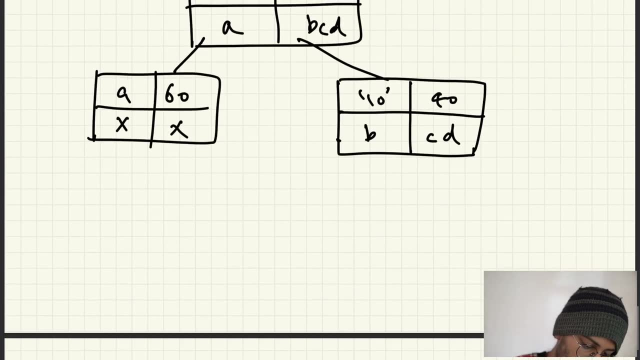 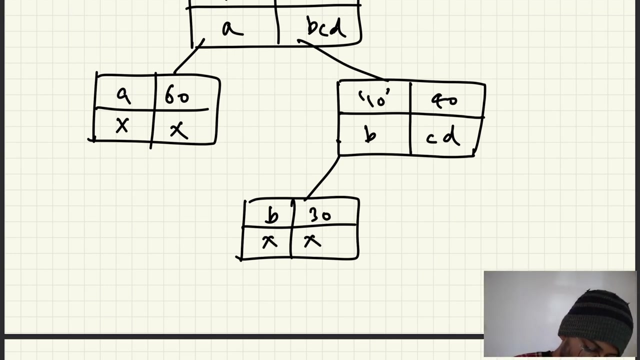 we know what B C D means here: 40 B and C D. what we know. we know we know what B C D means here: 40 B and C D. okay, then again B node, as it is, C D CD looks like this: okay, then again, B node as it is, C D CD looks like this: 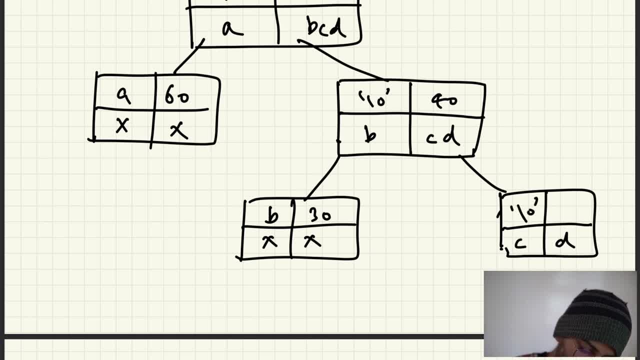 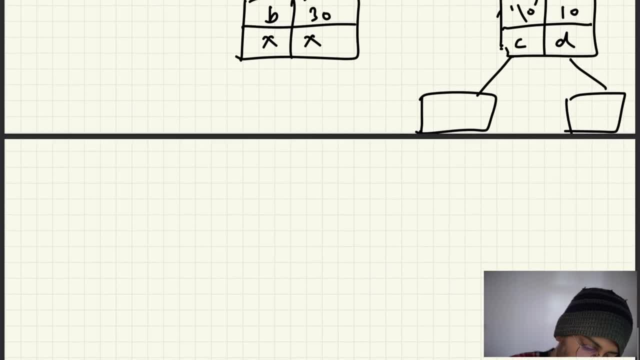 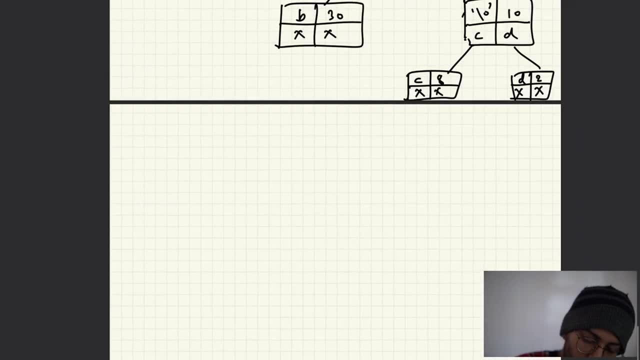 okay, then again B node, as it is, C, D, CD looks like this: C and D- nothing here. this was 10. then node C, node D: no D, nothing. this is what. C and D: nothing here. this was 10. then node C, node D: no D, nothing. this is what. 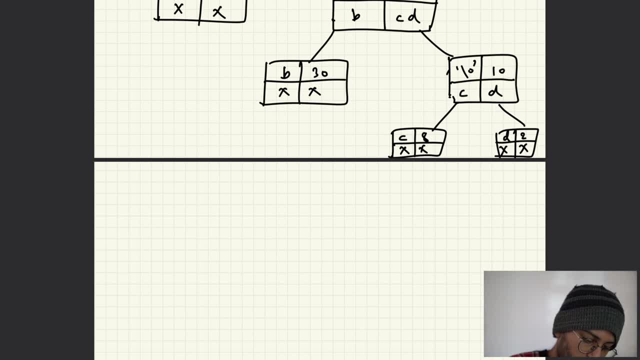 C and D: nothing here. this was 10. then node C, node D, no D, nothing. this is what it looks like my final tree. this is what it looks like my final tree. this is what it looks like my final tree. this is what my final tree looks like- easy nothing. 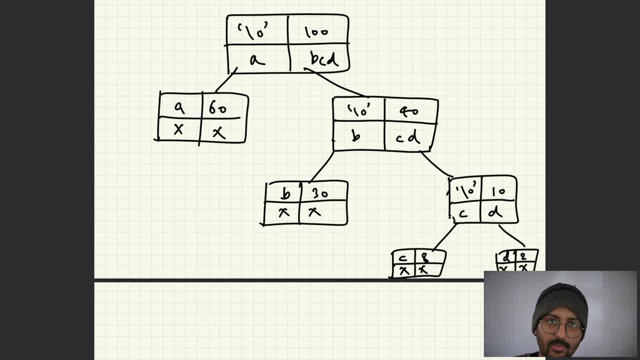 my final tree looks like easy nothing. my final tree looks like easy, nothing major. I've just taken a frequency, nothing major. I've just taken a frequency, nothing major. I've just taken a frequency. map step number one: I've listed. map step number one: I've listed. 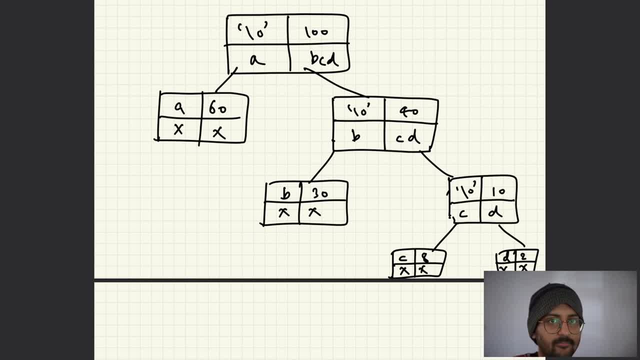 map, step number one. I've listed down steps as well. listed down steps as well. down steps as well. down steps as well. okay, so make the frequency map convert. okay, so make the frequency map convert. okay, so make the frequency map convert every key in the map into a node and put. 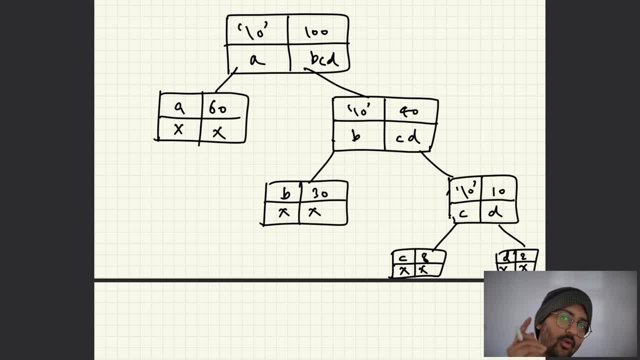 every key in the map into a node and put every key in the map into a node and put all those in a heap keep removing to and all those in a heap keep removing to and all those in a heap keep removing to and, as you keep removing, to combine and put. 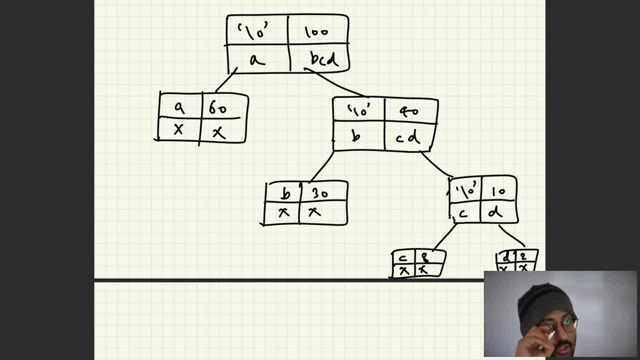 as you keep removing to combine and put, as you keep removing to combine and put it back in the heap. simple now. one more. it back in the heap. simple now. one more it back in the heap, simple now. one more thing is you need to do is when you move. 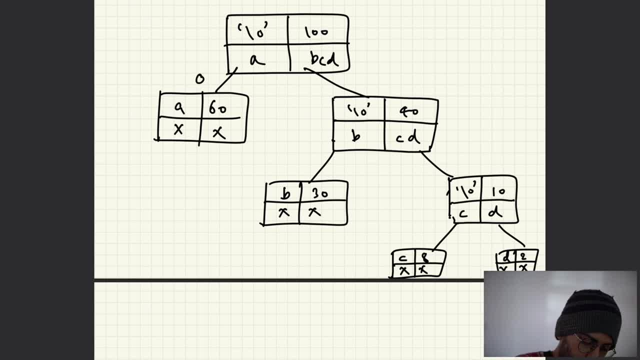 thing is you need to do is when you move thing is you need to do is when you move left. you have to add zero, so I will left. you have to add zero, so I will left you have to add zero, so I will start reading zero and I will go right. 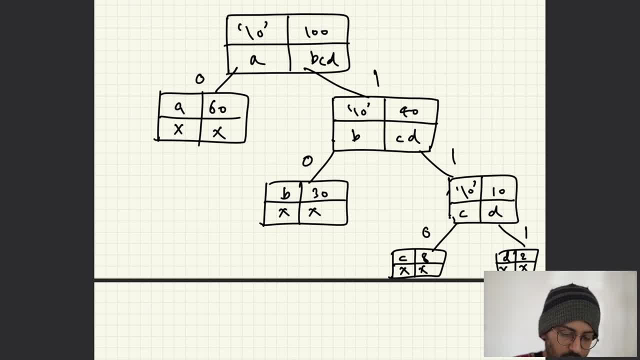 start reading zero, and I will go right. start reading zero and I will go right. one left, zero, right, one, zero one. so all one left zero, right, one, zero one. so all one left zero, right, one, zero one. so all the left you put zero, all the right you. 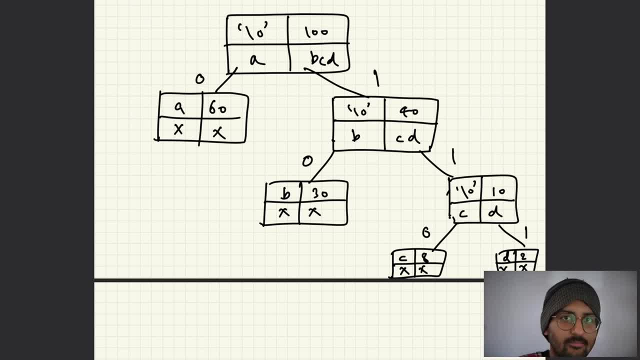 the left, you put zero, all the right. you the left, you put zero, all the right, you put one. don't ask why this is algorithm, put one. don't ask why this is algorithm, put one. don't ask why this is algorithm, for example. I'm like we do in linear. 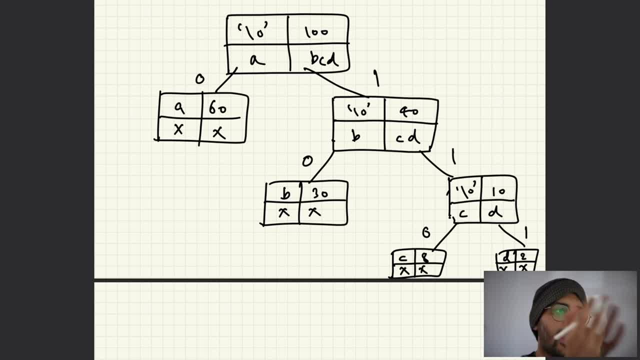 for example. I'm like we do in linear, for example. I'm like we do in linear search. we start searching from the first search. we start searching from the first search. we start searching from the first element. why in the binary search we have element. why in the binary search we have: 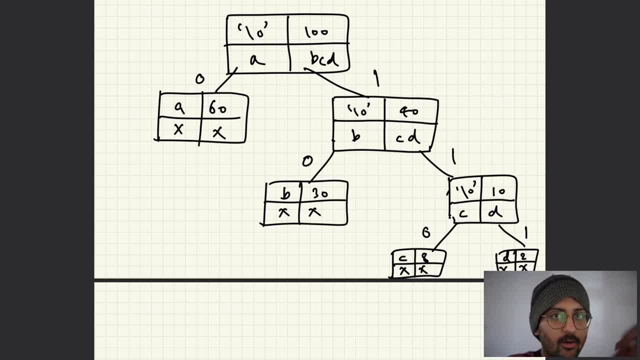 element. why, in the binary search, we have to cut it in middle? why? why do we need to cut it in middle? why? why do we need to cut it in middle? why? why do we need to do it? don't be that guy, don't be that- to do it. don't be that guy, don't be that. 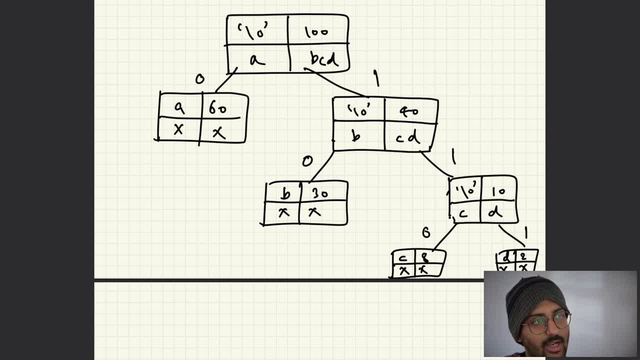 to do it. don't be that guy, don't be that student. here it's saying that left has student. here it's saying that left has student. here it's saying that left has to be zero. right has to be one. why what? to be zero right has to be one. why what? 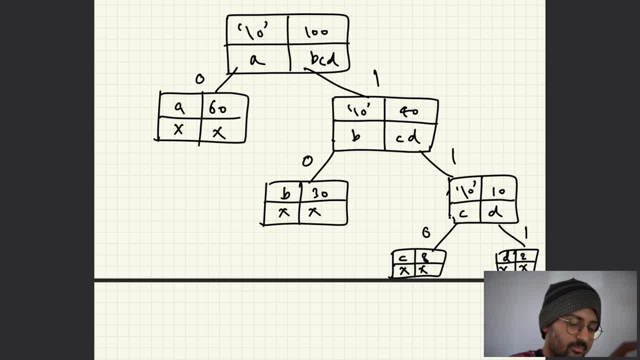 to be zero right has to be one. why, what do you mean? why it's the algorithm? do you mean why it's the algorithm? do you mean why it's the algorithm? someone created it with algorithm- okay. someone created it with algorithm- okay. someone created it with algorithm- okay, because that's how we're gonna use it. if 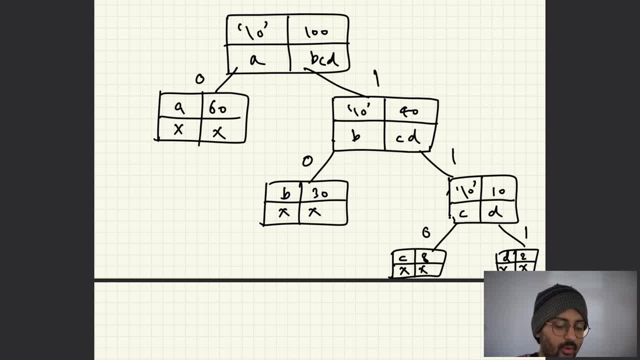 because that's how we're gonna use it. if, because that's how we're gonna use it. if you do want to know the reason behind it, you do want to know the reason behind it. you do want to know the reason behind it. it's so that we don't have- let me just it's so that we don't have. let me just it's so that we don't have. let me just show you the reason. so what we're going show you the reason, so what we're going show you the reason. so what we're going to do is we're going to retrieve the. 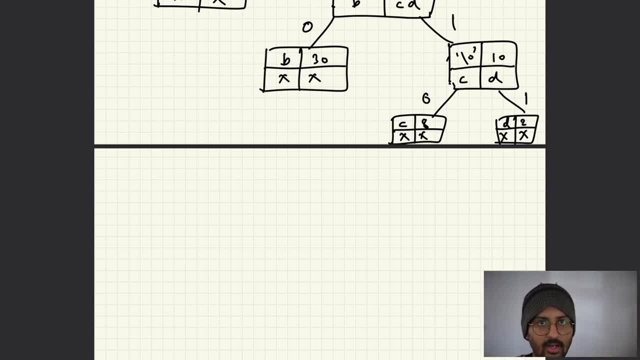 to do is we're going to retrieve the to do is we're going to retrieve the last node. okay, and we're going to pass last node. okay, and we're going to pass last node. okay, and we're going to pass the tree to fill the encoder and decoder. 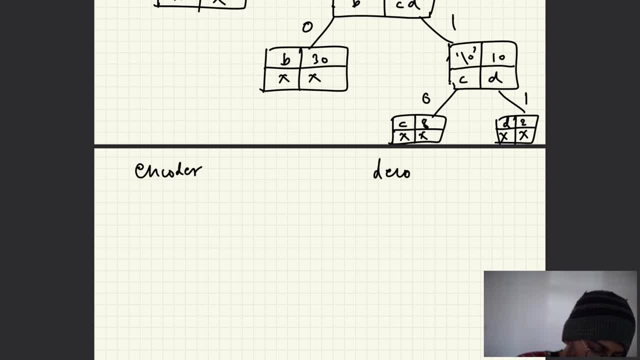 the tree to fill the encoder and decoder, the tree to fill the encoder and decoder. so my encoder and my decoder now I will. so my encoder and my decoder now I will. so my encoder and my decoder now. I will explain to you why we are doing zeros. 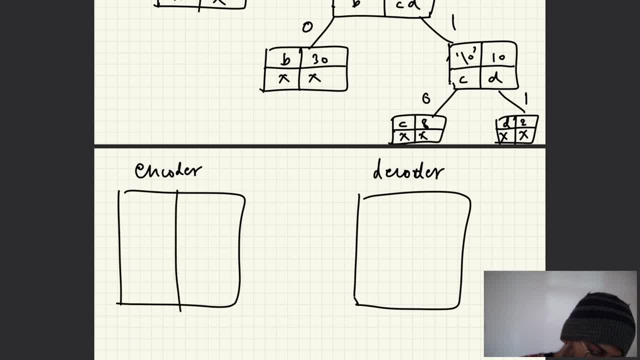 explain to you why we are doing zeros, explain to you why we are doing zeros and ones here and ones here, and ones here, ABCD, ABCD. okay. so here, if I say what is the ABCD, ABCD, okay. so here, if I say what is the? 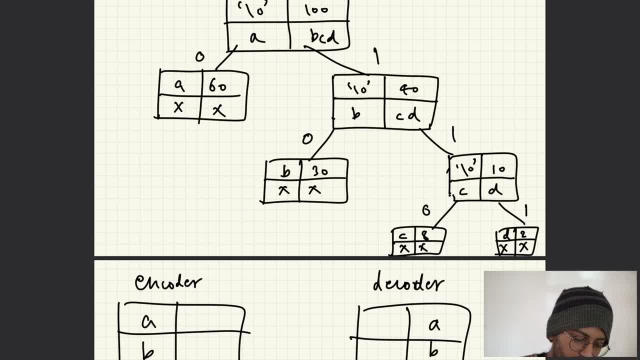 ABCD, ABCD. okay, so here, if I say, what is the value of a? the value of a is the path value of a. the value of a is the path value of a. the value of a is the path that takes, that takes, that takes it to reach from the main node root. 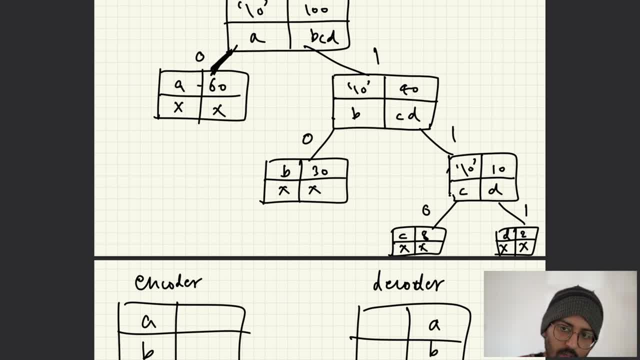 it to reach from the main node root it to reach from the main node root node to a root node to a path is just node to a root. node to a path is just node to a root. node to a path is just this one and it's only 0, so it will be. 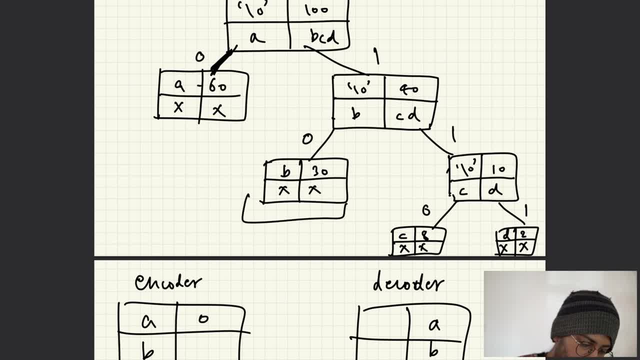 this one and it's only 0, so it will be this one and it's only 0, so it will be 0. what does it take to reach B? you tell 0. what does it take to reach B? you tell 0. what does it take to reach B? you tell me 1, 1, 0. B is 1, 0, C- C is from root. 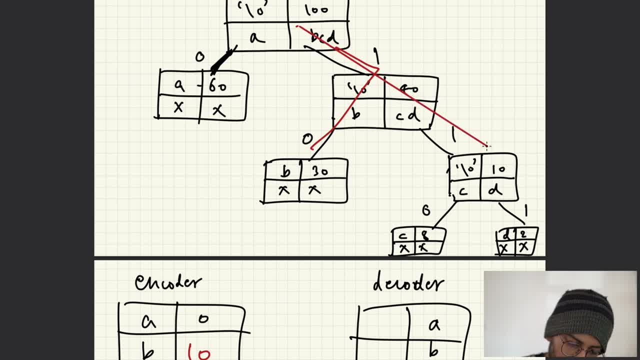 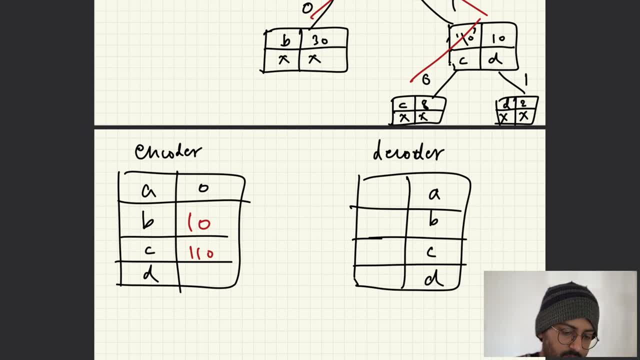 me 1 1 0 B is 1 0 C, C is from root me 1 1 0 B is 1 0 C, C is from root node 1 1 0. node 1 1 0. node 1 1 0 C. C is from root node 1 1 0, 1 1 0 and D is 1 1 1. 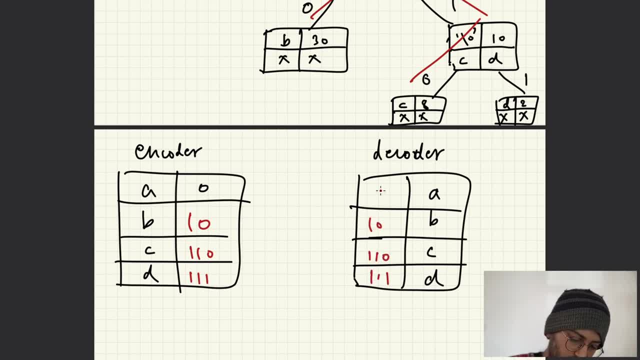 ok. 1 1 1, 1, 1, 1 0, 1 0 sounds good. this is ok: 1 1 1, 1. 1 1 0. 1 0 sounds good. this is ok. 1 1 1, 1, 1, 1 0, 1 0 sounds good. this is how we fold perform our encoder and. 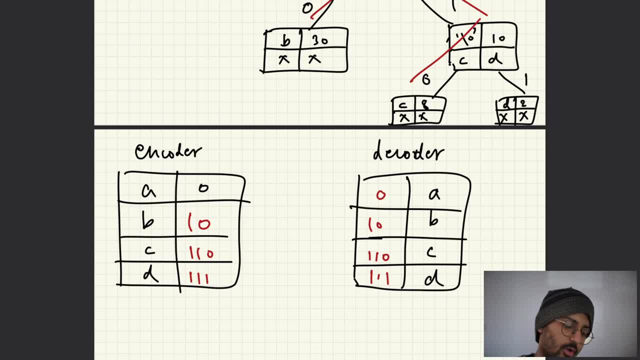 how we fold, perform our encoder and how we fold, perform our encoder and decoder hash maps. ok, Kunal, this is fine decoder hash maps. ok, Kunal, this is fine decoder hash maps. ok, Kunal, this is fine. every character that was in our main, every character that was in our main. 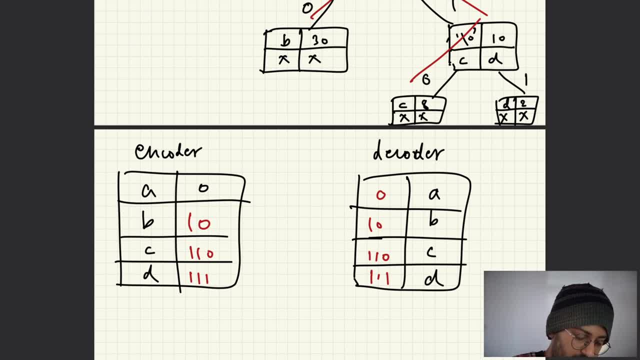 every character. that was in our main message that we want to send our friend message that we want to send our friend message that we want to send our friend has a different, has a different, has a different. value now in the form of ones and zeros. value now in the form of ones and zeros. 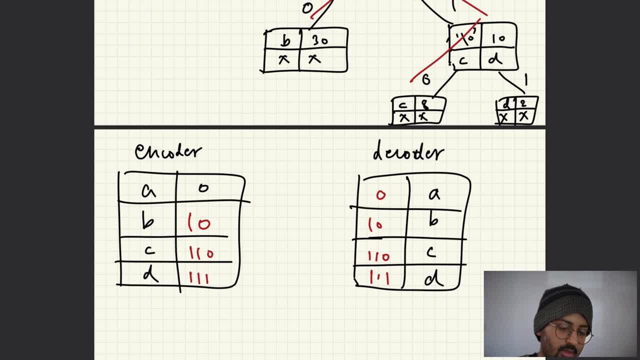 value now in the form of ones and zeros, because we know in reality, everything is. because we know in reality, everything is. because we know in reality, everything is boiled down to 1 and 0. this is fine. boiled down to 1 and 0, this is fine. 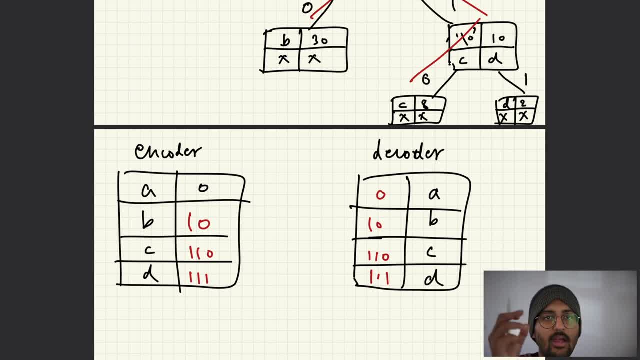 boiled down to 1 and 0. this is fine, Kunal, we can make this. it's easy. just Kunal, we can make this. it's easy. just Kunal, we can make this. it's easy. just create frequency map every node for every. create frequency map every node for every. 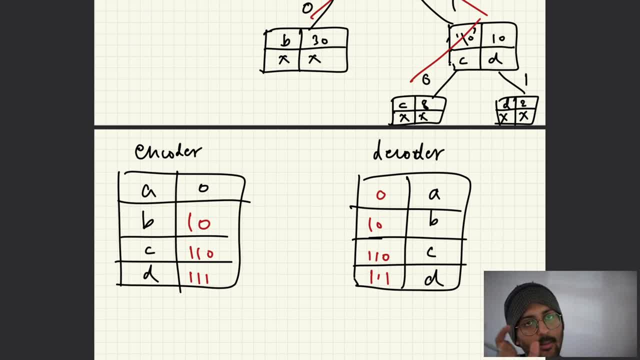 create frequency map, every node for every key in the map. put all those in a heap key in the map. put all those in a heap key in the map. put all those in a heap. take two out, combine those two, put it. take two out, combine those two, put it. 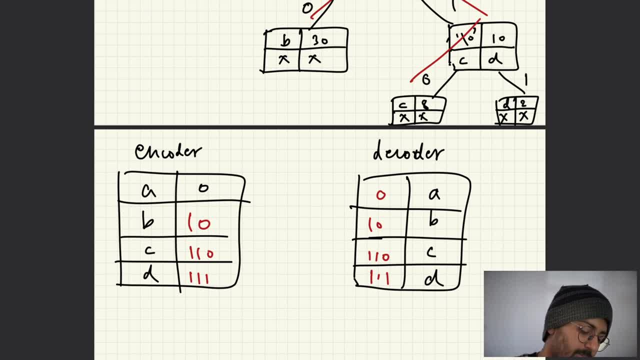 take two out, combine those two, put it back in. keep doing it till. one item is back in. keep doing it till. one item is back in. keep doing it till one item is for every character that is in the, for every character that is in the, for every character that is in the string. but how is it going to help us? 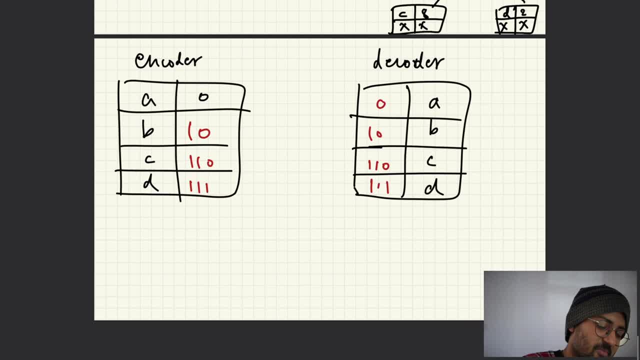 string, but how is it going to help us? string, but how is it going to help us? some reduce the size and encode and some reduce the size and encode and some reduce the size and encode and decode. let's see now. now, let's see the decode. let's see now. now, let's see the. 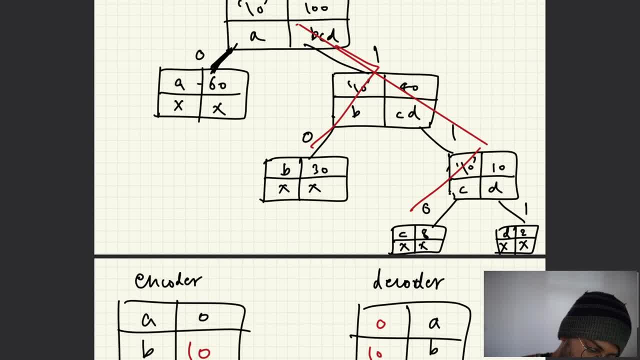 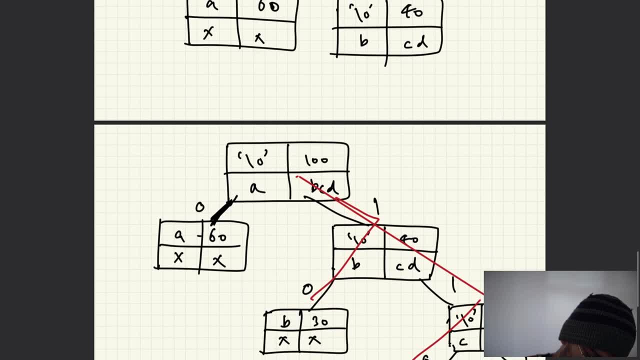 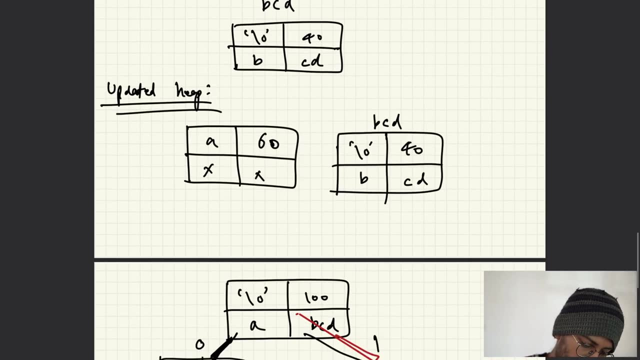 decode. let's see now. now let's see the magic, magic, magic so step number. forgot to write the steps four. was this: step number four, step number. step number four, step number. step number four, step number. this last one, here i can say five. this last one, here i can say five. 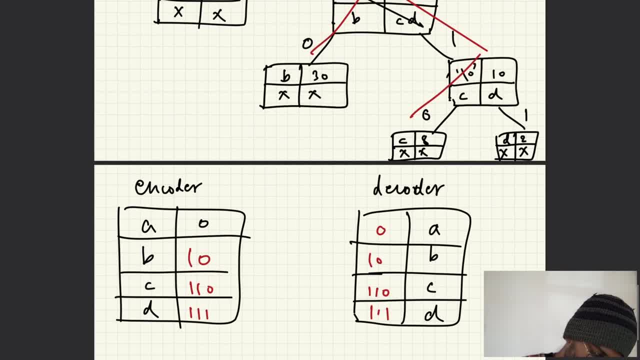 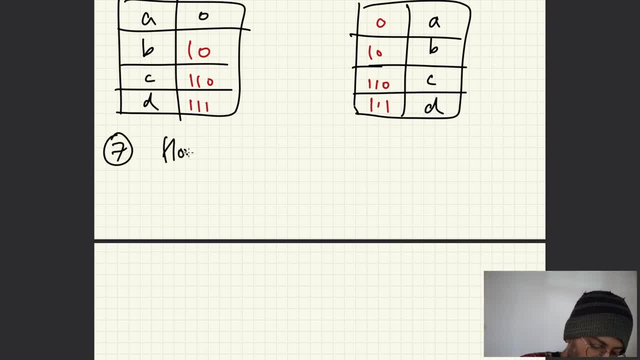 this last one. here i can say five, this one, this one, this one, six step number seven. six step number seven. six step number seven. how to encode and decode. so let's say the string is the message. so let's say the string is the message. so let's say the string is the message. you're saying your friend is. 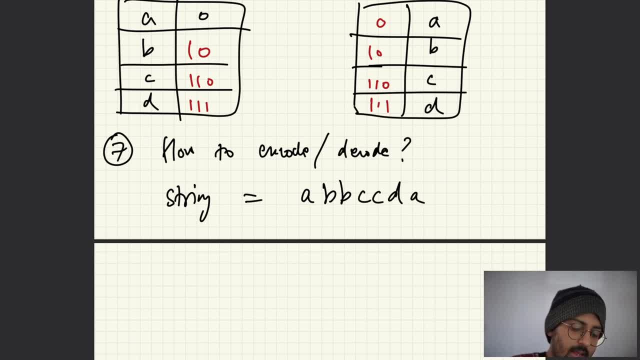 you're saying your friend is. you're saying your friend is a, b, b, c, c, d, a. suppose that is the message: a, b, b, c, c, d, a. suppose that is the message: a, b, b, c, c, d, a. suppose that is the message you're sending, your friend. 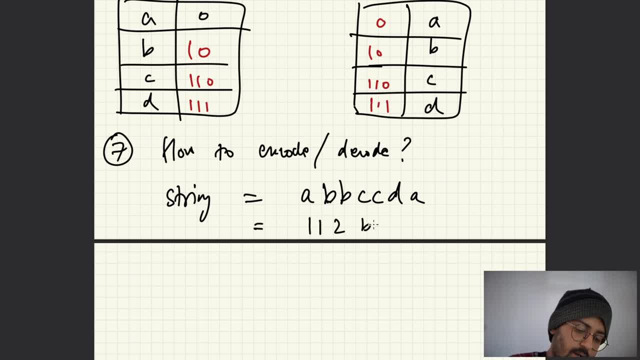 you're sending your friend. you're sending your friend. okay, let's take an example. and this is okay. let's take an example and this is okay. let's take an example, and this is: i know 112 bits because seven into two. i know 112 bits because seven into two. 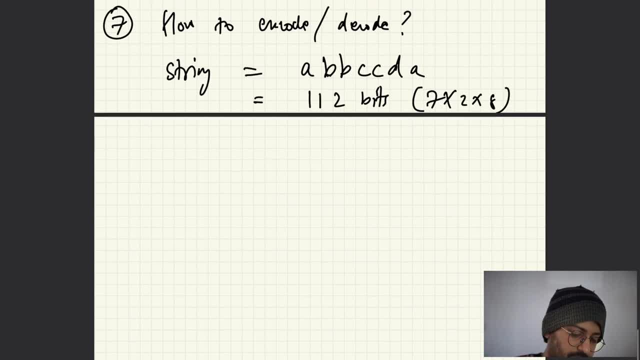 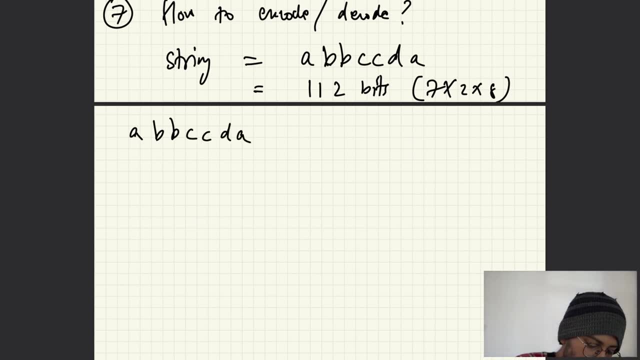 i know 112 bits, because seven into two bytes into eight bits, bytes into eight bits, bytes into eight bits. okay so if i write a, b, b, c, d a. okay so if i write a, b, b, c, d a. okay so if i write a, b, b, c, d a, a, b, b, c, c, d a. 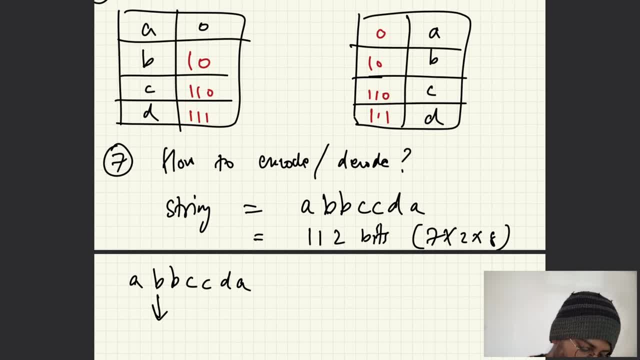 a, b, b, c, c, d, a, a, b, b, c, c, d, a. if i write it, replace it using the. if i write it, replace it using the. if i write it, replace it using the. encoder map a is 0. encoder map a is 0. encoder map a is 0. d is 1: 0. again, b is 1: 0. c is 1: 1, 0. 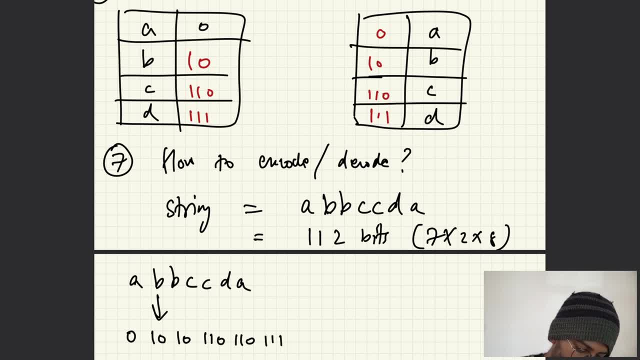 d is 1 0, again b is 1 0, c is 1 1 0, d is 1 0 again, b is 1 0, c is 1 1 0 again. c 1 1 0, d is 1 1, 1 and a is again 0. again: c 1 1 0 d is 1 1, 1 and a is again 0. again c 1 1 0 d is 1 1, 1 and a is again 0. how much, how many bits are these? 1, 2, 3, 4? 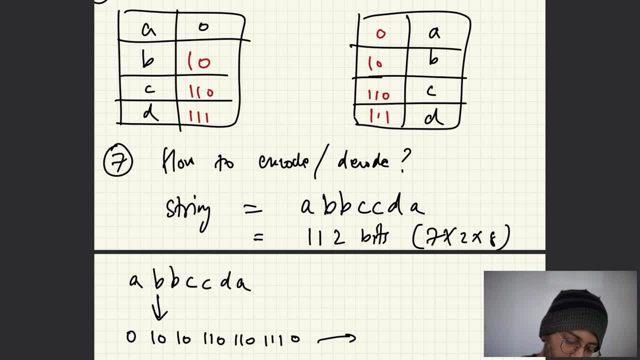 how much? how many bits are these? 1, 2, 3, 4. how much? how many bits are these? 1, 2, 3, 4, 5, 6, 7, 8, 9, 10, 11, 12, 13, 14, 15 bits. 5, 6, 7, 8, 9, 10, 11, 12, 13, 14, 15 bits. 5, 6, 7, 8, 9, 10, 11, 12, 13, 14, 15 bits. so we saved the original message in 15. 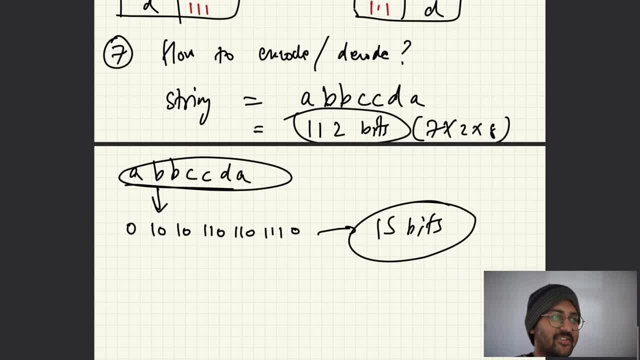 so we saved the original message in 15. so we saved the original message in 15 bits instead of 112 bits. bits instead of 112 bits. bits instead of 112 bits. compression, compression, compression, nice, nice, nice. now, how do we make this using this, uh? 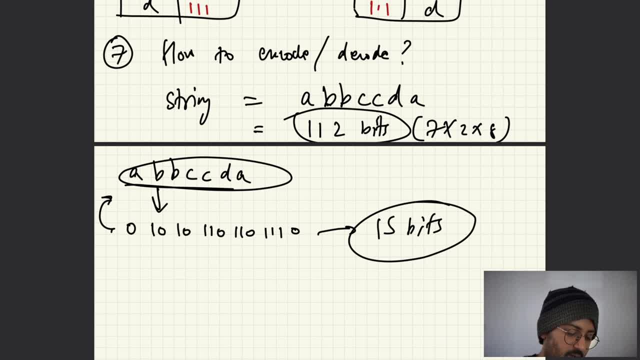 now, how do we make this using this? uh. now, how do we make this using this? uh, series of bits. how do you make the series of bits? how do you make the series of bits? how do you make the original message? you check a, you check. original message. you check a, you check. 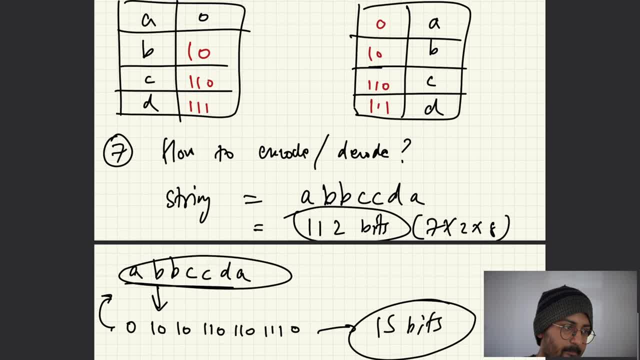 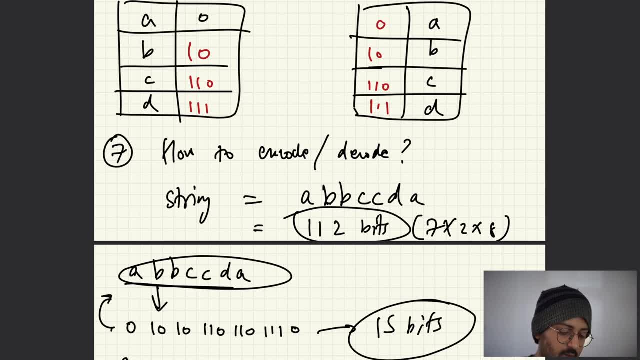 original message. you check a. you check for zero. is zero existing in the in the encoder? yes, i will do a check for in the encoder. yes, i will do a check for in the encoder. yes, i will do a check for one one existing. no one zero existing. 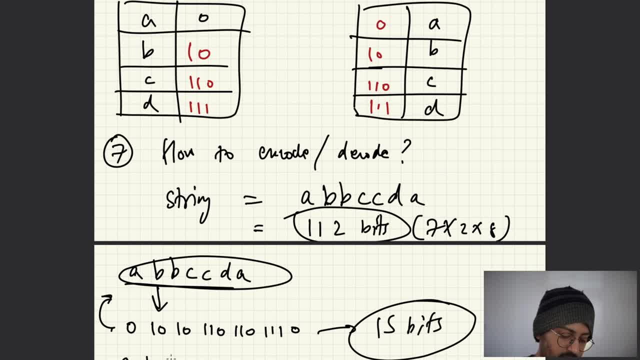 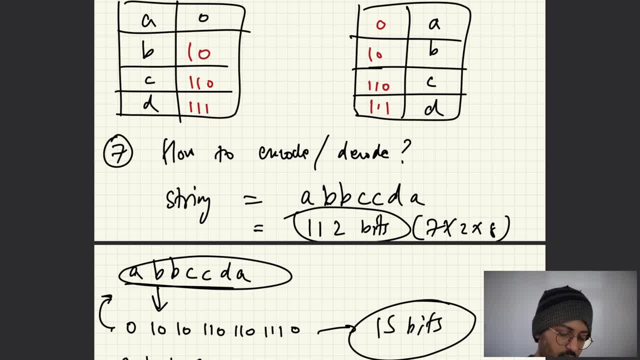 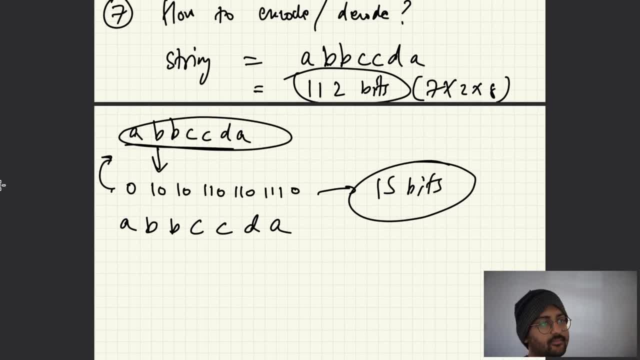 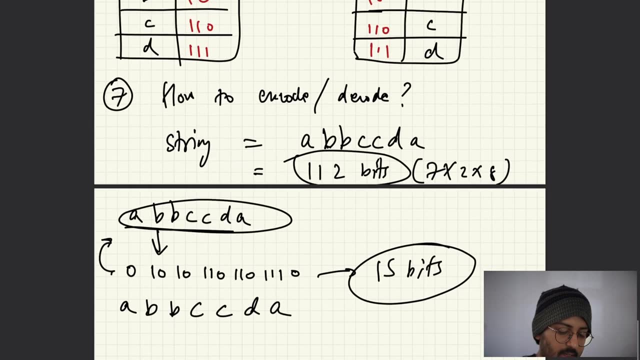 one, one one existing, yes, zero existing. yes, one one one existing. yes, zero existing. yes, there you go. how cool is that? okay? so the question is: you'll be like, okay. so the question is: you'll be like, okay. so the question is: you'll be like kunal, what if some other 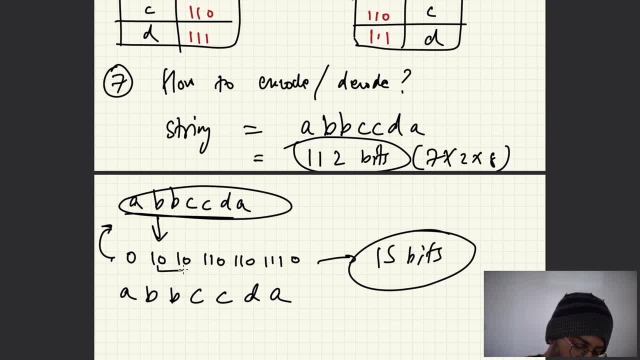 kunal. what if some other kunal? what if some other the. the doubt that people the. the doubt that people the. the doubt that people have is kunal. what if there's some other have is kunal? what if there's some other have is kunal? what if there's some other sequence of characters here, like zero one? 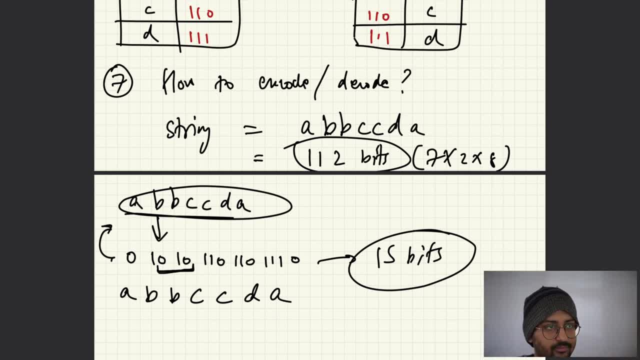 sequence of characters here like zero. one sequence of characters here like zero one zero. why is it not checking for zero zero? why is it not checking for zero zero? why is it not checking for zero one zero? this is not happening because our tree. this is not happening because our tree. 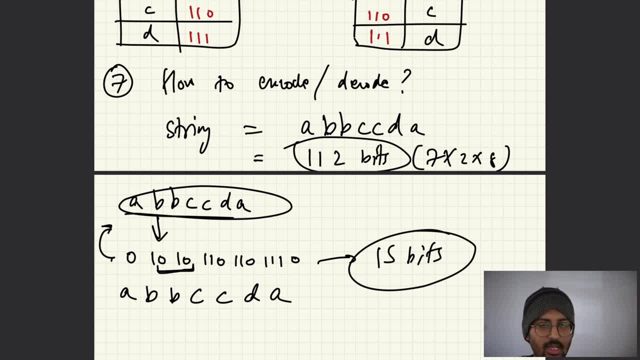 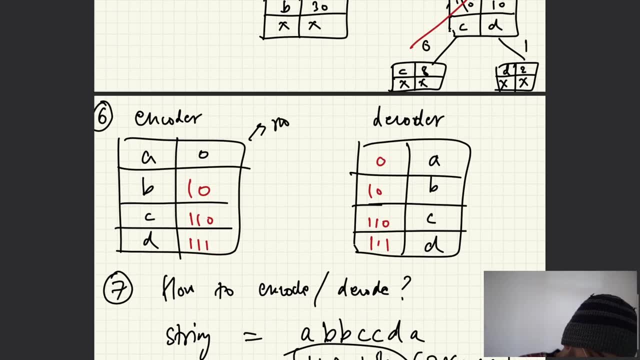 this is not happening because our tree is making sure, is making sure, is making sure that the value- any value- is not a that the value- any value is not a that. the value- any value- is not a prefix of the next value, prefix of the next value, prefix of the next value. here you can see: 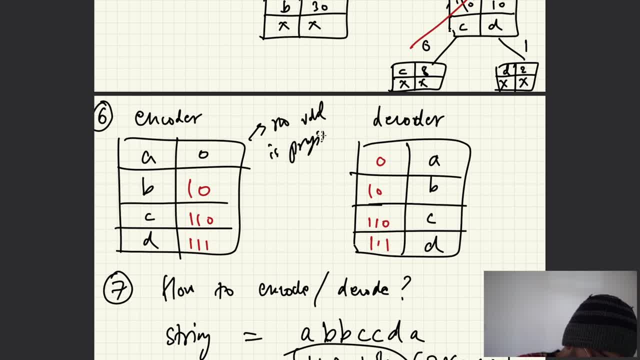 here you can see, here you can see no value, no value. no value is prefix of, is prefix of, is prefix of another value. so if a is a is going to be zero, then so if a is a is going to be zero, then so if a is a is going to be zero, then there is no other value that has. 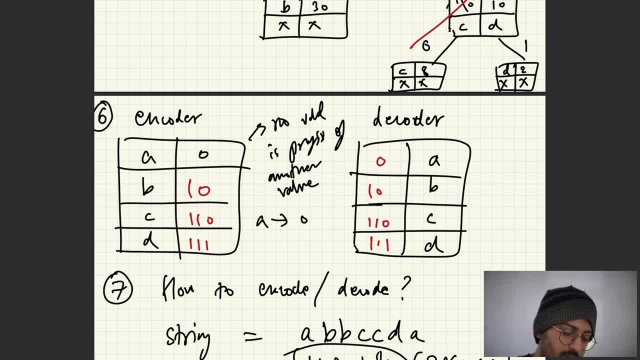 there is no other value that has. there is no other value that has starting zero. if the value of b is starting zero, if the value of b is starting zero, if the value of b is 10, there is no other value that has 10. there is no other value that has. 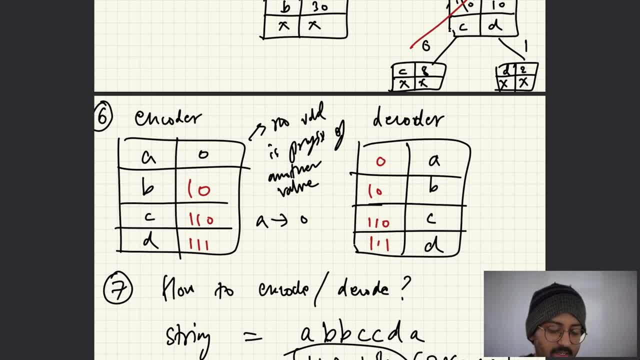 10. there is no other value that has starting as 10.. starting as 10.. starting as 10.. if the value of c is 110, there is no. if the value of c is 110, there is no. if the value of c is 110, there is no other value is starting at 110. 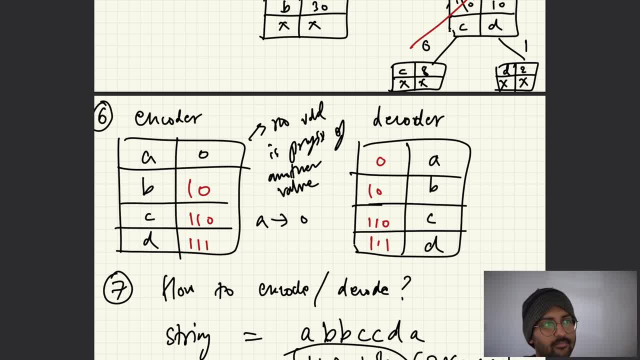 other value is starting at 110, other value is starting at 110, so on and so forth. make sense, make sense, make sense. that is how it makes sure you may have, that is how it makes sure you may have. that is how it makes sure you may have. this doubt, kunal, what if there's? 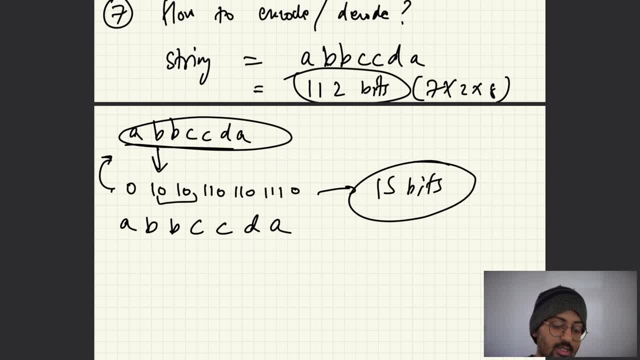 this doubt kunal? what if there's this doubt kunal? what if there's some other thing in the middle like 010, some other thing in the middle like 010, some other thing in the middle like 010, or 101, no, or 101, no. 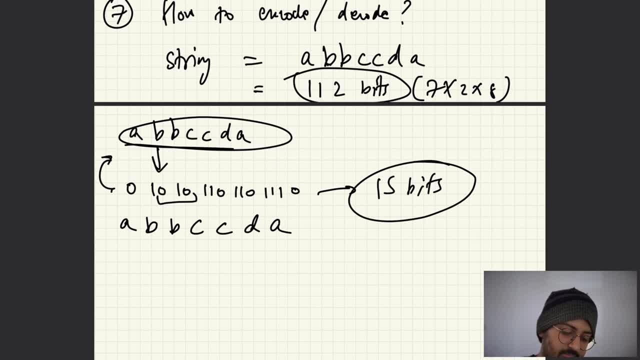 or 101. no, so 15 bits instead of using 112. you're so 15 bits instead of using 112. you're so 15 bits instead of using 112. you're using 15 bits. using 15 bits. using 15 bits. okay, okay. 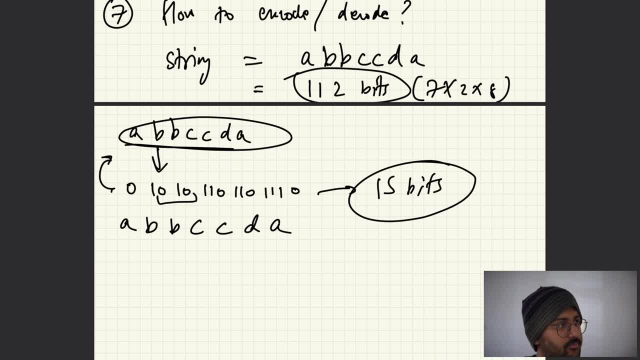 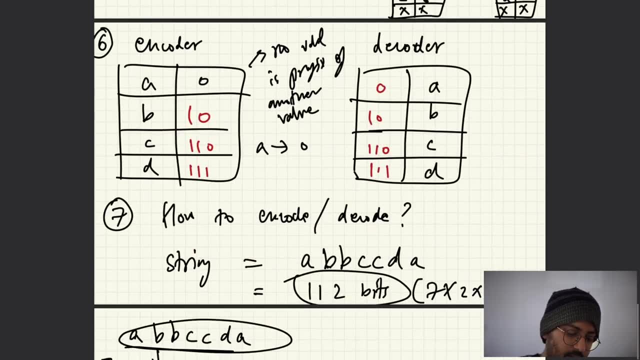 okay, sounds good, sounds good, sounds good. cuckoo, cuckoo, cuckoo. space complexity is what space complexity is what space complexity is what to store it in the map and stuff that to store it in the map and stuff that to store it in the map and stuff that i'm creating. this is very easy. 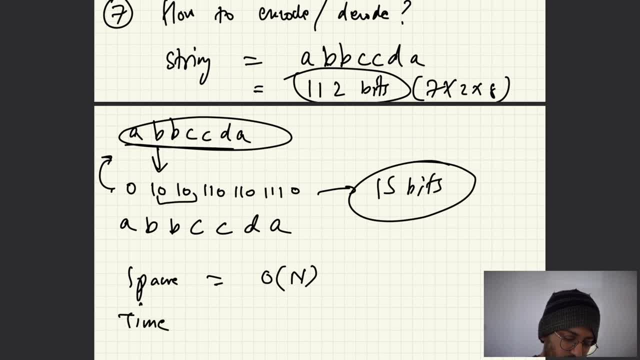 we go off n, but the question is time we go off n, but the question is time we go off n, but the question is time. complexity is what? let's say there are n nodes. what is the? let's say there are n nodes? what is the? let's say there are n nodes? what is the time? complexity? 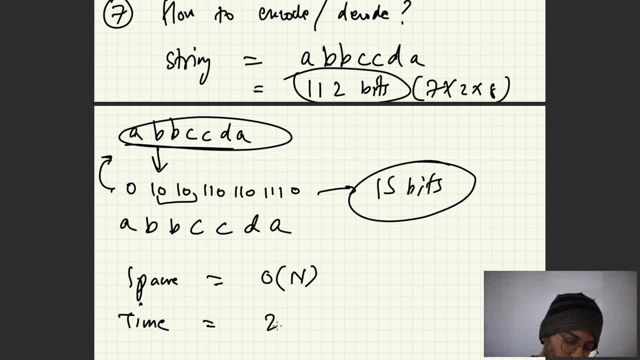 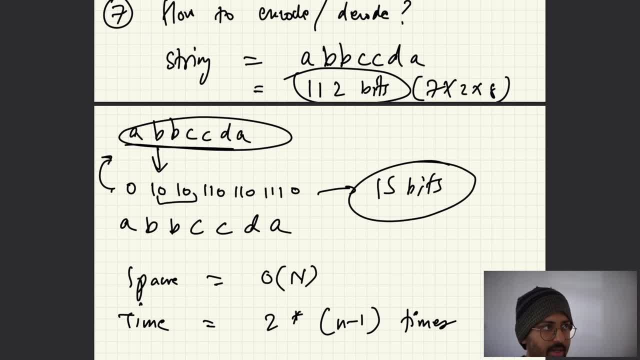 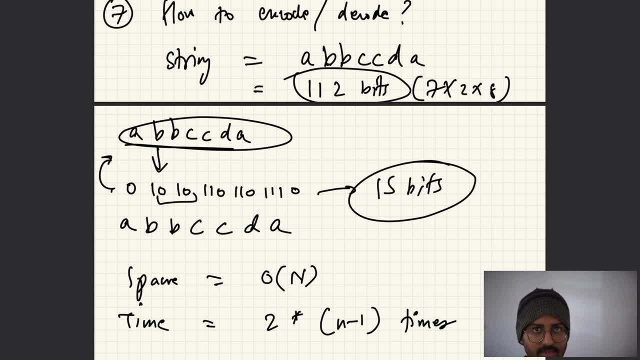 okay, or 2 n times, whatever you want to okay, or 2 n times, whatever you want to call it. if you want to be specific, you call it. if you want to be specific, you call it. if you want to be specific, you can do 2 into n minus 1 times. 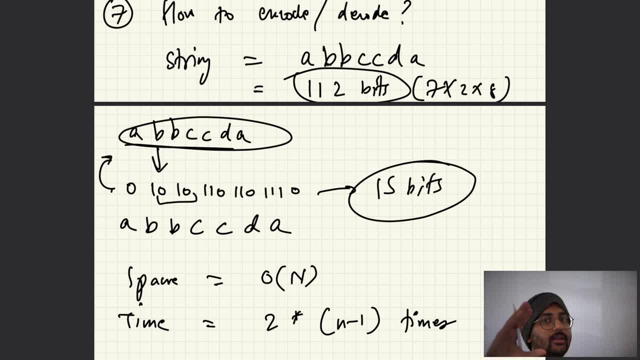 can do 2 into n minus 1 times. can do 2 into n minus 1 times, because the first node, because one node, because the first node, because one node, because the first node, because one node will always remain in the heap right, will always remain in the heap right. 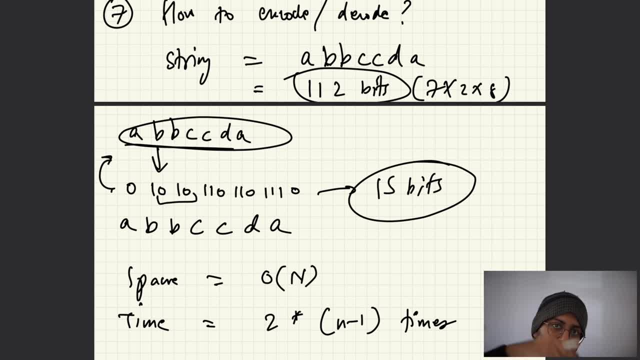 will always remain in the heap right. you are not removing that last node. you are not removing that last node. you are not removing that last node. that's why n minus 1 and you're doing. that's why n minus 1 and you're doing. that's why n minus 1 and you're doing every operation twice. 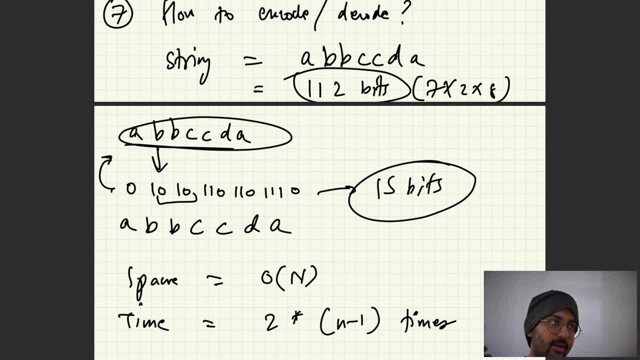 every operation twice. every operation twice. and what is the cost to remove an element and what is the cost to remove an element, and what is the cost to remove an element or an insert, an element or an insert, an element or an insert, an element into the heap. 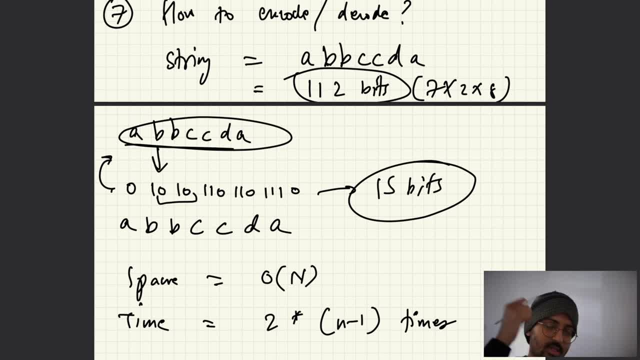 this is actually insertion and removal. this is actually insertion and removal. this is actually insertion and removal. right, you're first inserting, then you're right, you're first inserting, then you're right, you're first inserting, then you're removing, removing, removing. so twice for every element, but not the. 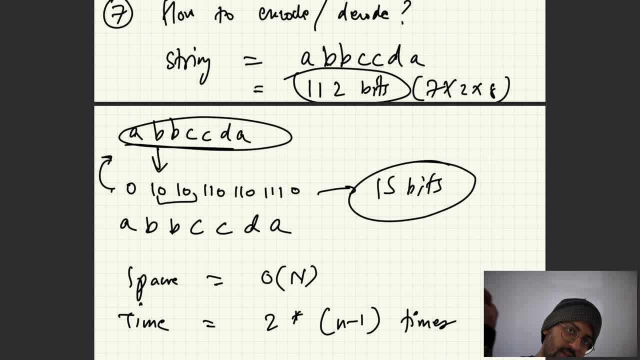 so twice for every element, but not the. so twice for every element, but not the very first element. very first element, very first element. what is the cost for every insertion, or what is the cost for every insertion, or what is the cost for every insertion or deletion in the heap log of n? 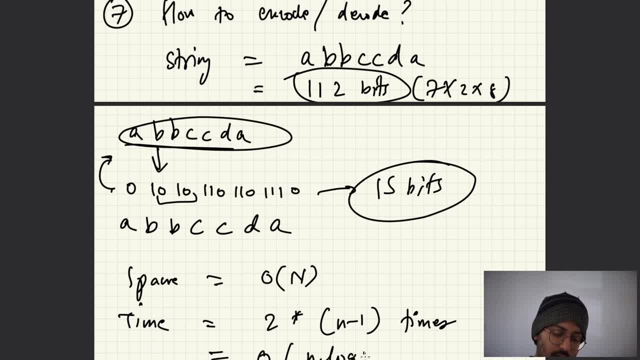 deletion in the heap log of n. deletion in the heap log of n. time complexity. is n log n. log of n into 2 into n minus 1 constants. log of n into 2 into n minus 1 constants. log of n into 2 into n minus 1 constants removed. 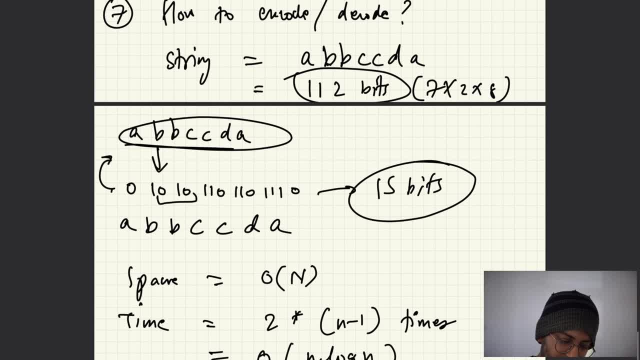 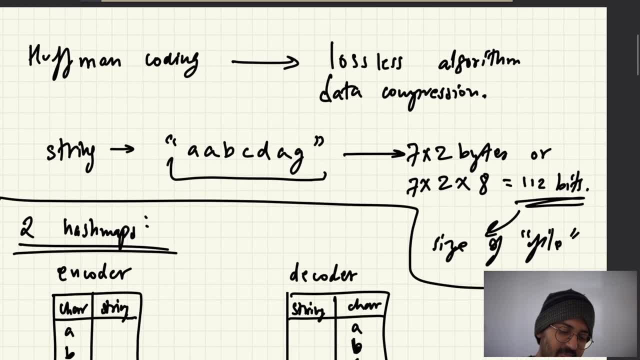 removed. removed o of n log n. that's it. that's huffman coding, and that's it. that's huffman coding, and that's it. that's huffman coding. and decoding, decoding, decoding- easy it is very easy, easy it is very easy, easy it is very easy. but now we're going to code it, so let's. 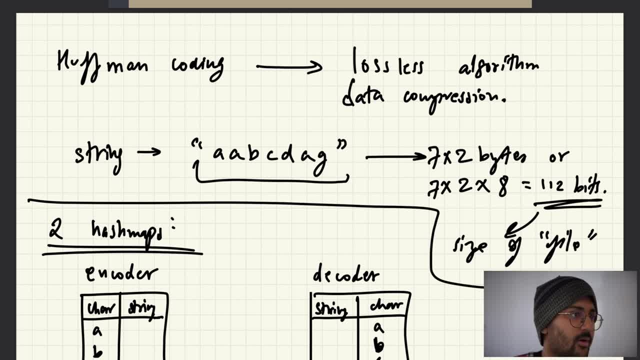 but now we're going to code it, so let's. but now we're going to code it, so let's code it, code it, code it. by the way, code can be found in the. by the way, code can be found in the. by the way, code can be found in the description below. okay, so here i have my. 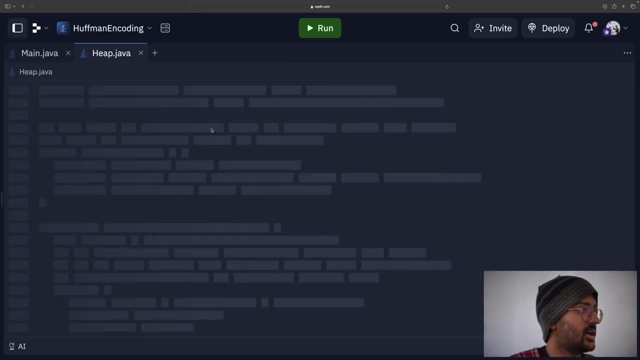 description below: okay, so here i have my description below. okay, so here i have my file. and also, since we're using heap file, and also since we're using heap file, and also since we're using heap, we have done heaps before check out the. we have done heaps before check out the. 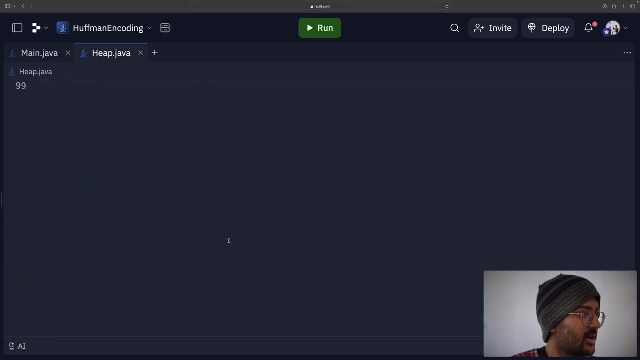 we have done heaps before. check out the video. and i showed you how to video and i showed you how to video and i showed you how to create this entire heap function. so create this entire heap function. so create this entire heap function. so, uh, not the function, the class, so your. 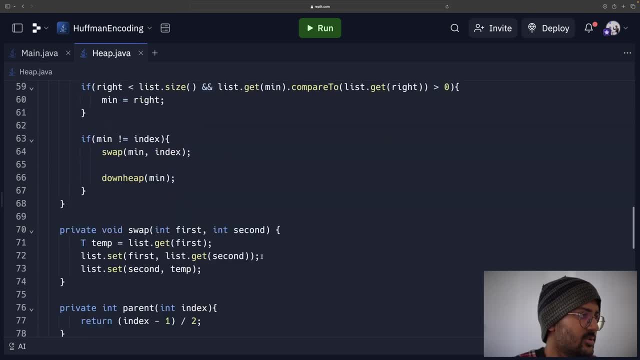 uh, not the function the class. so your, uh, not the function, the class. so your own heap class priority queue, whatever own heap class priority queue, whatever own heap class priority queue, whatever, you can use the inbuilt one as well. you can use the inbuilt one as well. 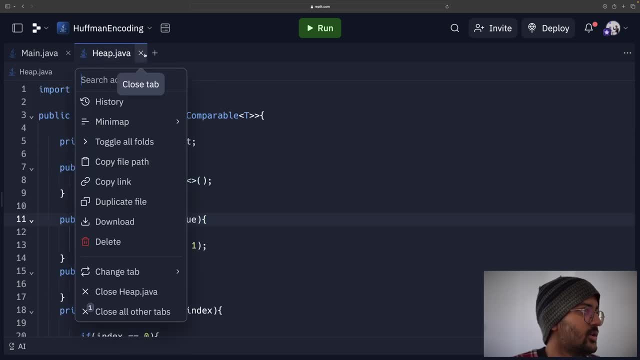 you can use the inbuilt one as well, but i'm just going to use the one i, but i'm just going to use the one i, but i'm just going to use the one i created in previous lectures, created in previous lectures, created in previous lectures so you can watch the previous lecture. 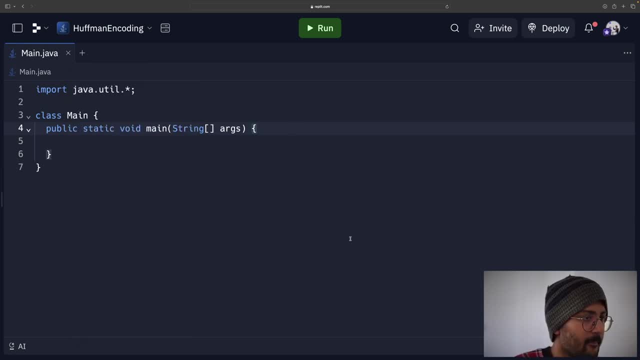 so you can watch the previous lecture. so you can watch the previous lecture if you want to learn more about how heaps, if you want to learn more about how heaps, if you want to learn more about how heaps work internally and everything work internally and everything work internally and everything but we're going to create. 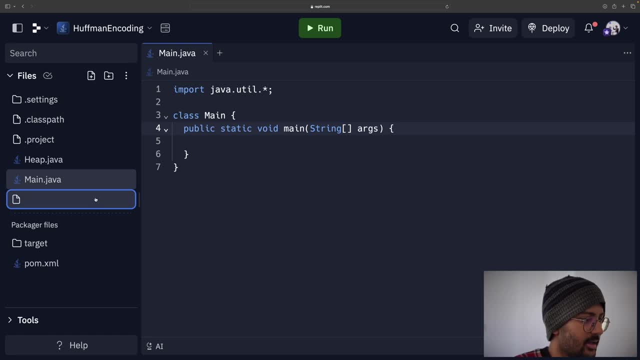 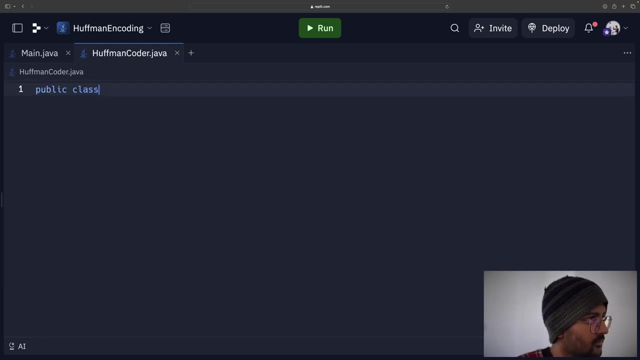 but we're going to create. but we're going to create huffman coder. so let's say i'll create a huffman coder. so let's say i'll create a huffman coder. so let's say i'll create a new file: huffman coderjava. 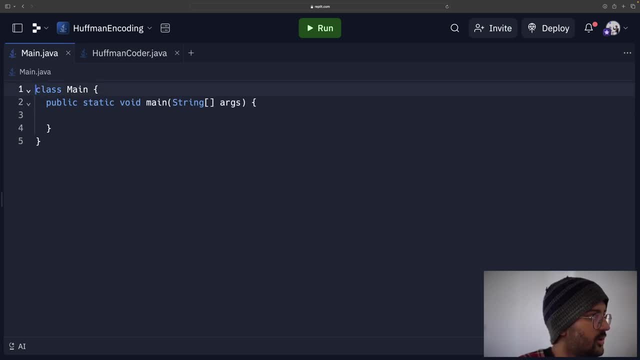 and i am going to use, because we're going to use hash map map, because we're going to use hash map map, because we're going to use hash map map, set all sorts of things, set all sorts of things, set all sorts of things. okay, so what do we need to do? 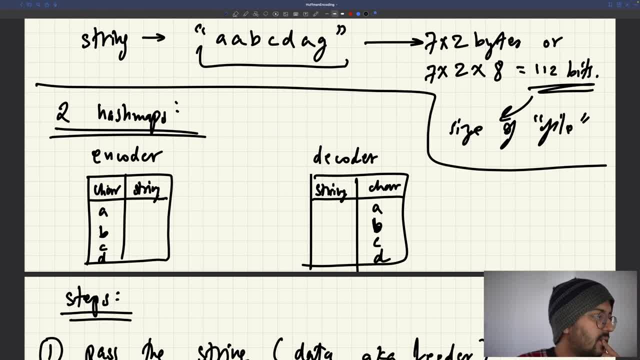 okay, so what do we need to do? okay, so what do we need to do? i need two hash maps, one encoder, one. i need two hash maps, one encoder one. i need two hash maps: one encoder, one decoder. the key of encoder is character. decoder: the key of encoder is character. 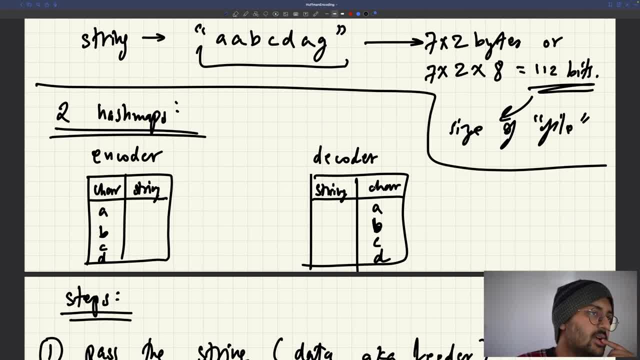 decoder, the key of encoder is character value string and for decoder, value is value string and for decoder value is value string and for decoder value is character key string, not a problem. i can. character key string, not a problem. i can. character key string, not a problem. i can do that. 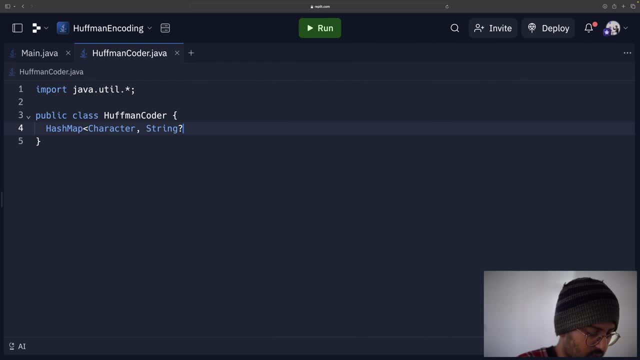 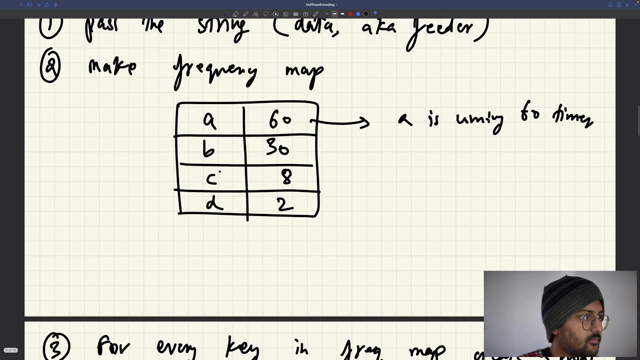 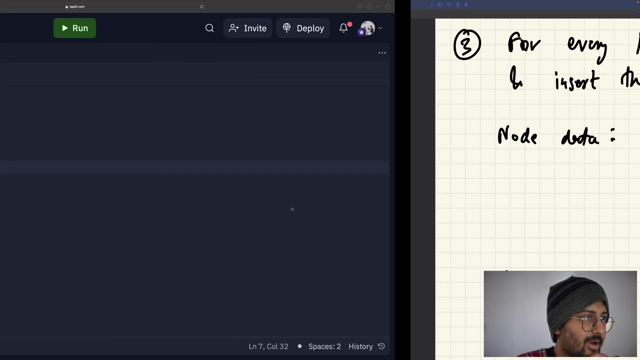 do that, do that hash map. this is, this is. this is encoder. this is encoder, this is decoder. I'm going to create a node. What does node contain? It is my node. Data cost left and right, And I want to compare two nodes as well, so I'll implement comparable. 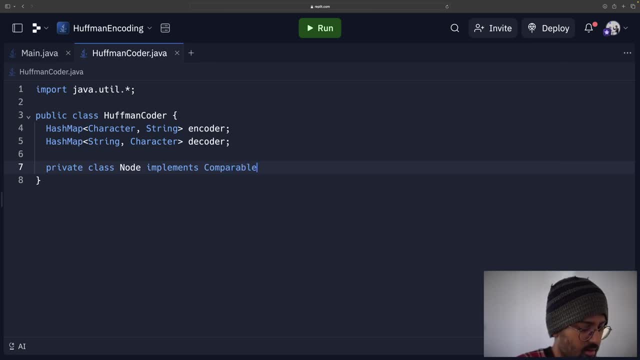 Now you'll be like Kunal: what is this? implements, comparable. Please don't ask me weird questions. What's the object? environment playlist. You're learning about hash maps and you're asking me what is implements in Java. No, not cool Generics and implements and stuff. Read what's the object. 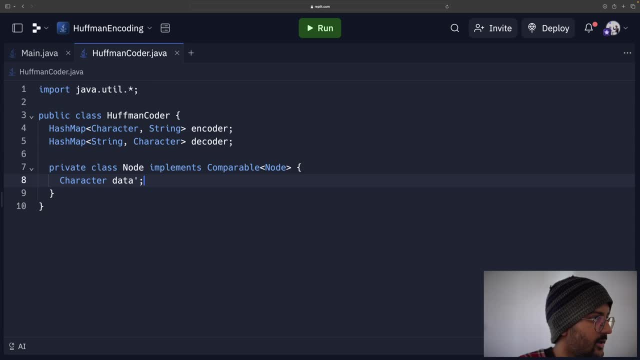 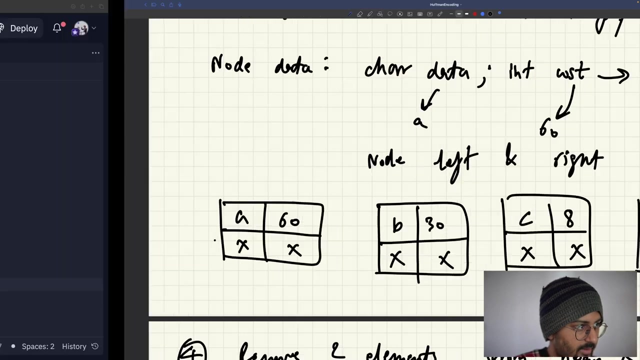 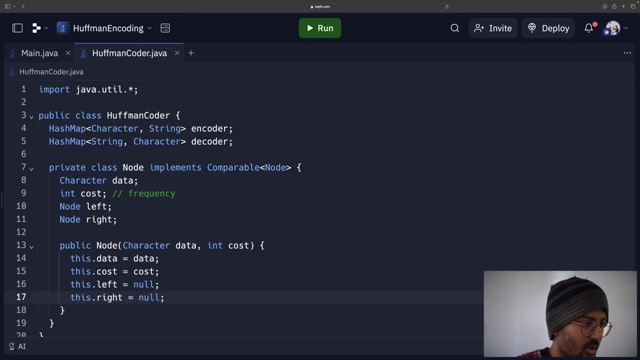 environment, playlist, Character data. I'll take the wrapper class. I'll have the cost. I'll have the node left and node right. This is nothing but frequency. Okay, Constructor, When a new node is added, And, And initially when a new node is added, this is fine, but the left and right are NULL. 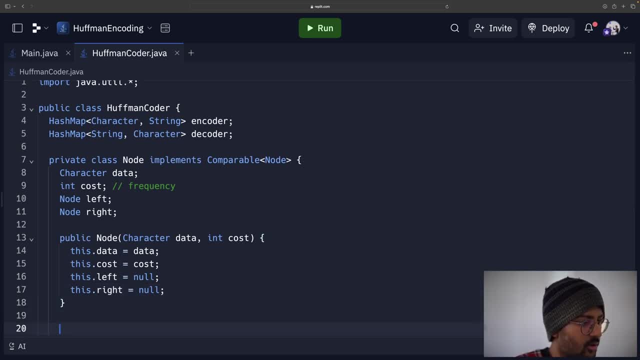 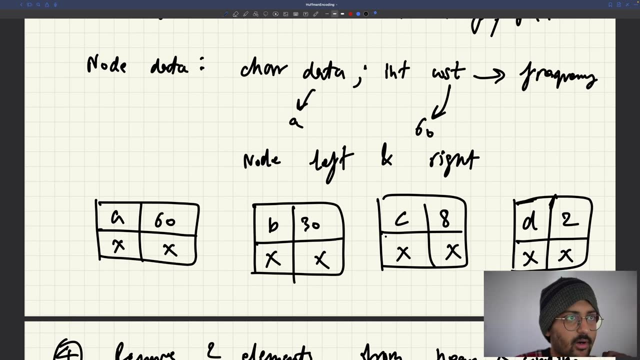 That looks good. And when we want to compare two nodes, I want to compare two nodes for MinHeap. So we were telling us, it was telling us that it's a MinHeap, so in the MinHeap it's going to be like it's taking the lowest value, the lowest value of what? 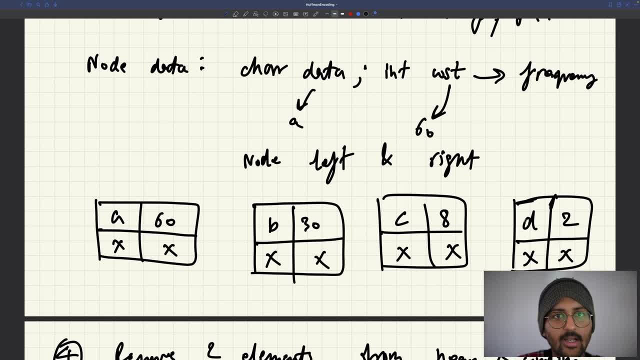 This node has four values: character: an integer, a left and a right. On which basis do you want me to say? I know you're saying: take the lowest in the basis of cost, like minimum heap or priority queue, based on what? 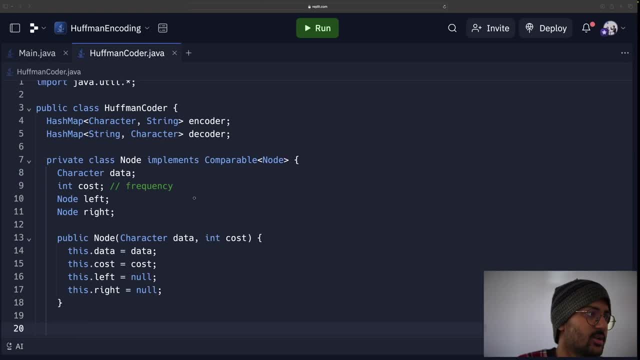 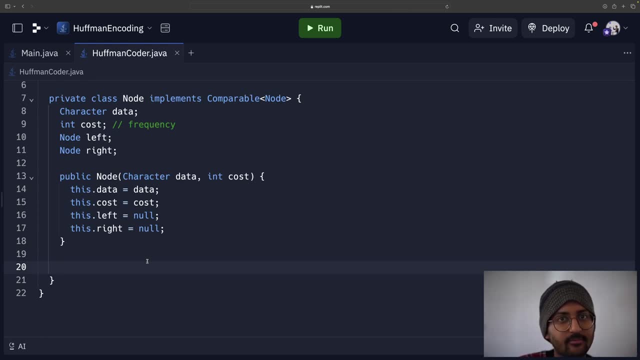 Based on the string or the character or the number, the number. So that's why I have to implement MinHeap, And the question for you is: which method do I have to override? Which method do I have to override in order to do this? compared to method. 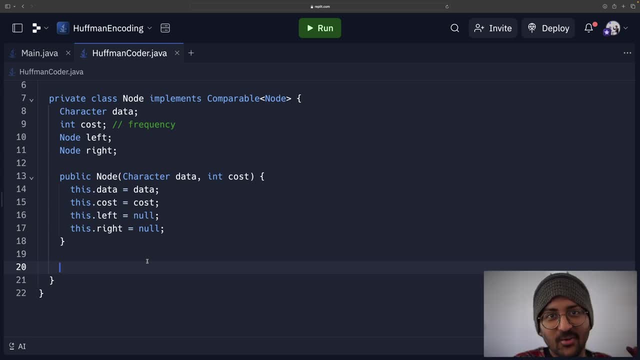 I'll do a reminder for you. Okay, I know I can, I can sense it, you know, through the camera, when there are there are some students have no idea about object-oriented programming, no idea about inheritance, no idea about overriding functions, anything. they have no idea, no clue. 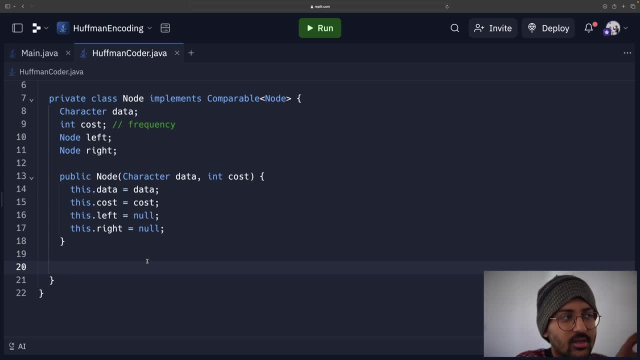 And then they start commenting and asking questions: Why have not you watched the object-oriented programming Playlist? That's my question. So if you're given, let's say, type node, okay, And you're given node A and node B, you're you're like, is node A greater than node B? 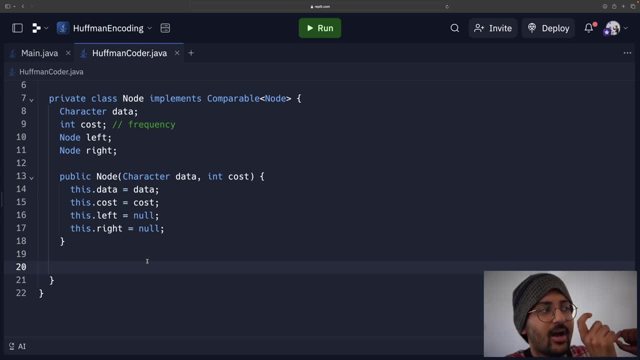 Java will get confused. What do you mean? Which property of node do you want me to compare when you're saying: is node A greater than node B? Do you want to compare the string of the node? Do you want to compare the integer of the node or the marks, whatever? whatever you. 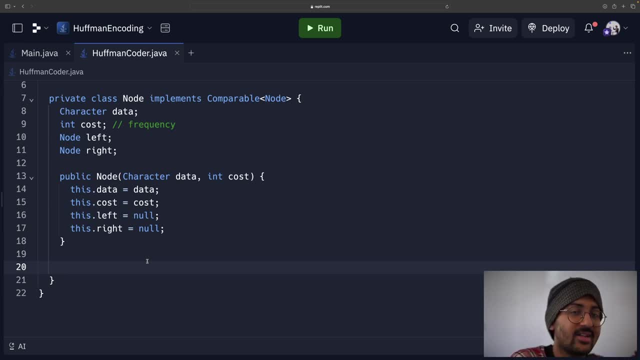 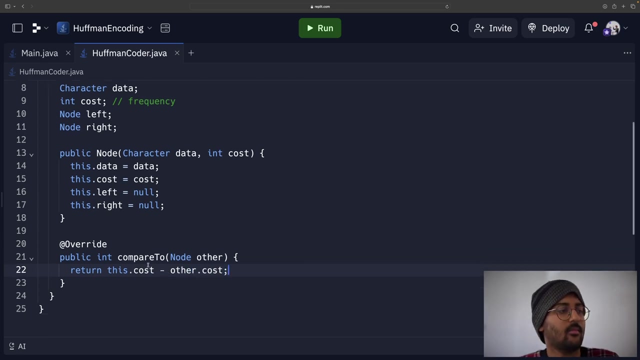 have. Let's see if it's a student node. So you have to explicitly tell it using the override method, the override annotation, by overriding the compare to method, I'm going to override based on cost. okay, You all know right. 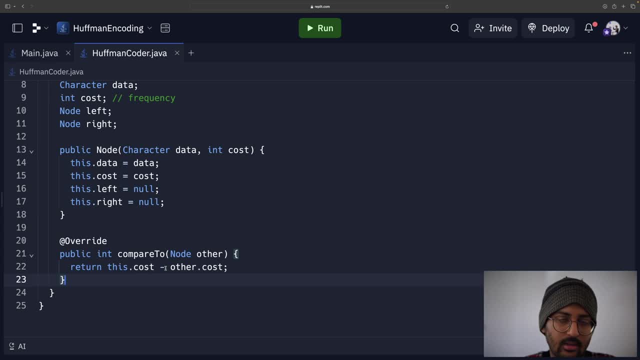 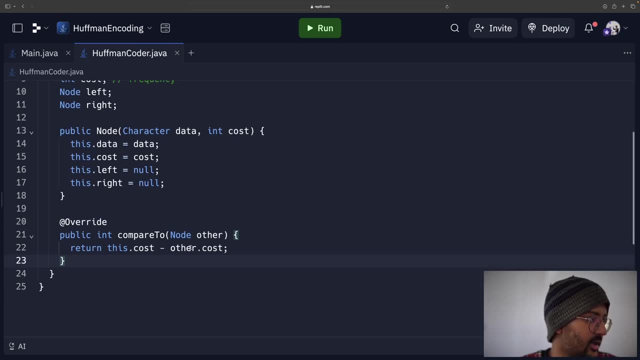 When? when it returns, negative means it's smaller. Uh, positive means bigger. Zero means both are equal. Very simple stuff. Why are you getting confused with, like, just watch, object-oriented programming list? Okay Now, constructor, I'll pass my string and it may throw an exception. 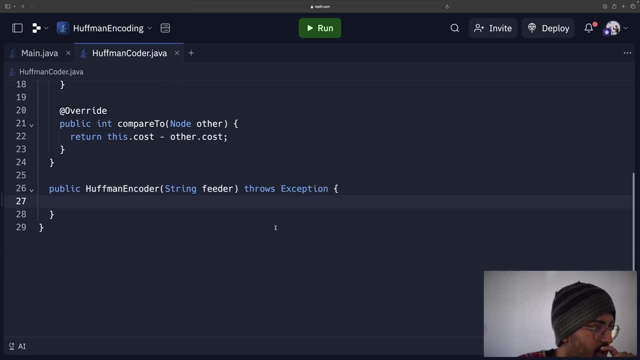 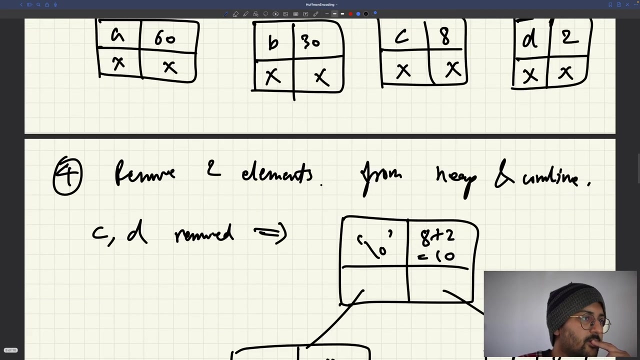 Okay, This is my constructor. Over here And in the constructor only, I will do everything. So when a new string, when a string is passed to me, I want to do some stuff. Okay, I want to encode and decode, but I want to form this entire tree in the constructor only. 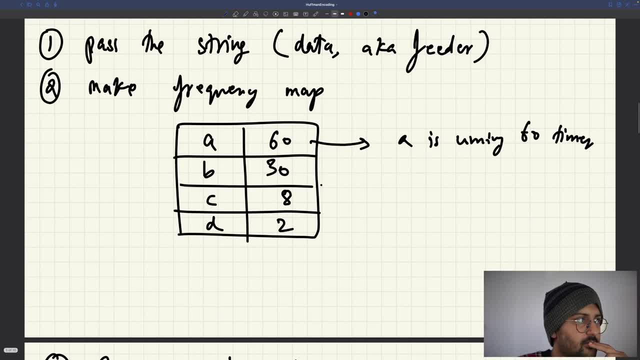 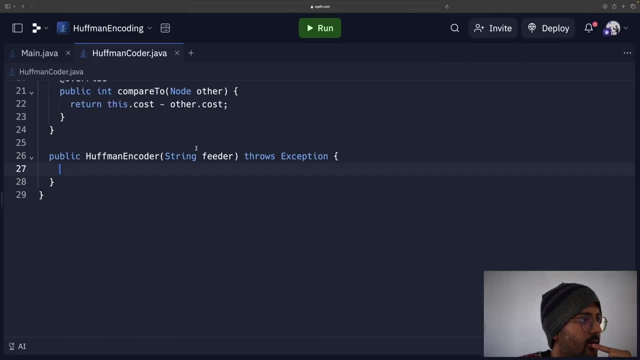 So how do we do that? Just read the notes that I have written: Pass the string. pass the string, make the frequency map. Not a problem. I will not even think. I will just do what the what the PDF says that I have over here. 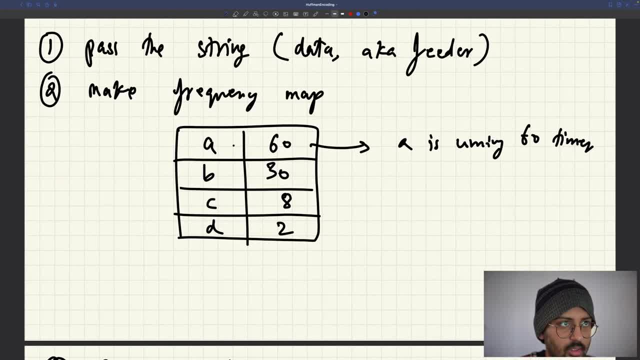 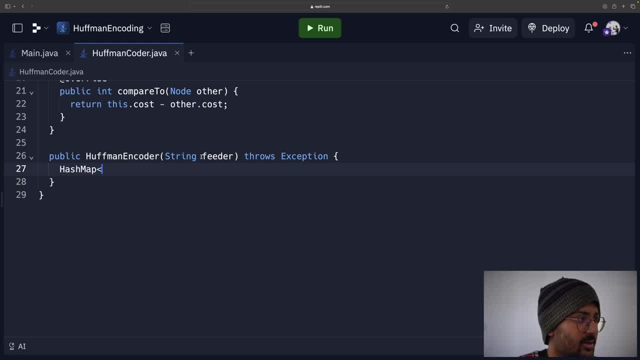 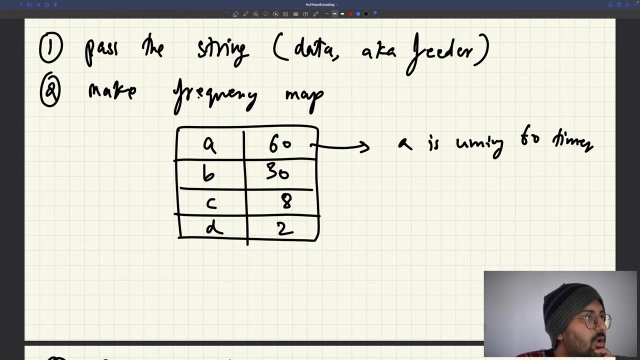 in the notes, This one, what's it called Good notes. But yeah, you will find the PDF of this written notes in the description as well. Character integer: frequency map is equal to new batch map. Okay, I have to create frequency map for every character in the string. 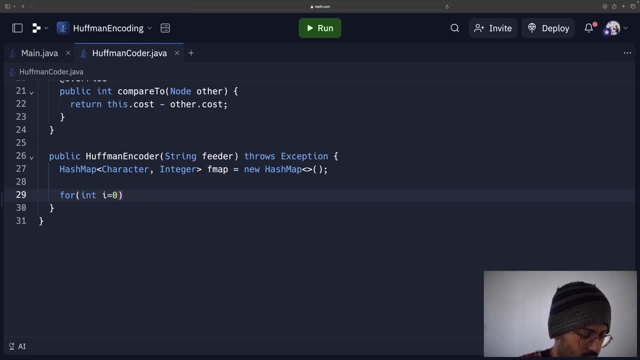 Not a problem. Character is what For every character. I'll write it in simple terms. Okay, If the map contains, I can write it in one line, but I'm writing it in every single step. So you know. but I should not, because previous lectures we have already covered how to create. 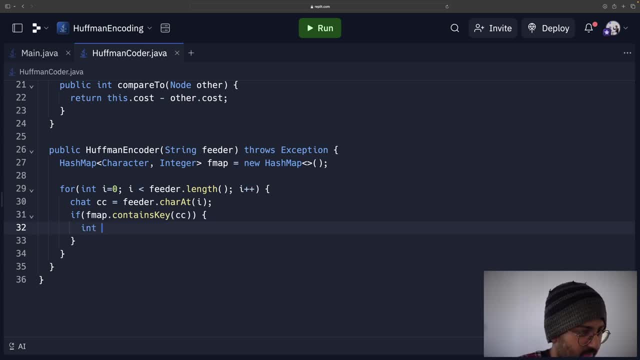 frequency map in hash maps. So yeah, I can say original value. I'm really doing it too much. Get the original value that already exists. Okay, So the character already exists. then just increase the original value plus one and put it in the map. 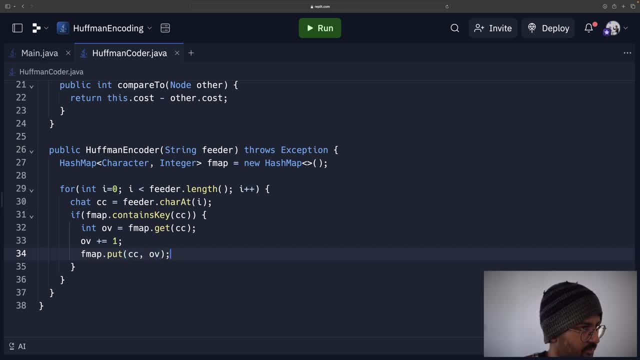 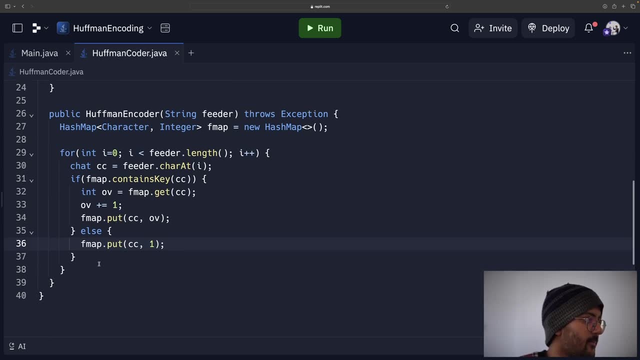 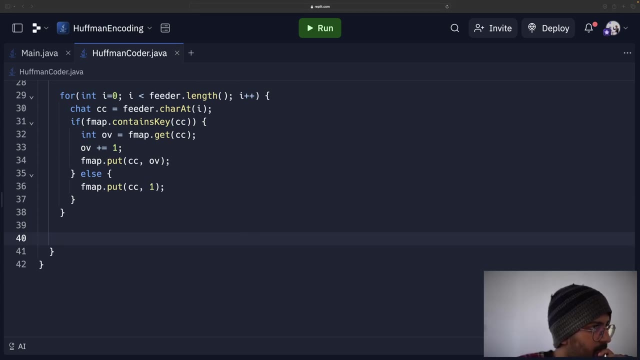 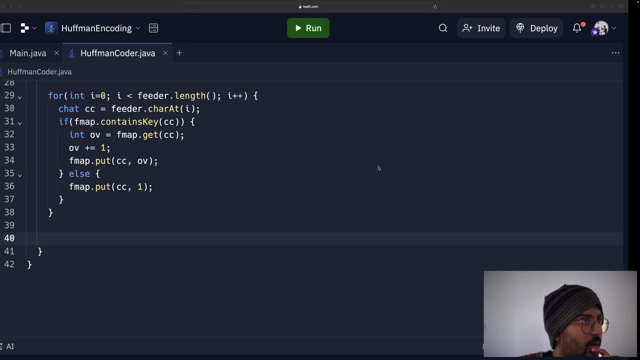 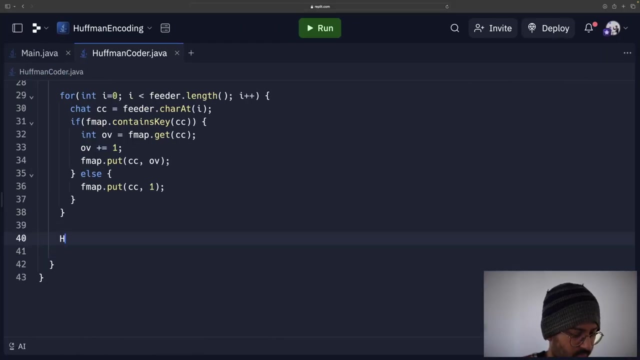 Character: original value. If it does not exist, put one. This is the first time I'm getting it. This will create me my frequency map. Okay, Sounds good, Cool Now. next step is creating the min heap. Okay. 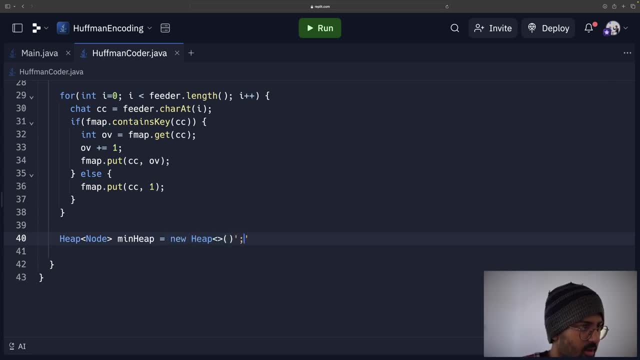 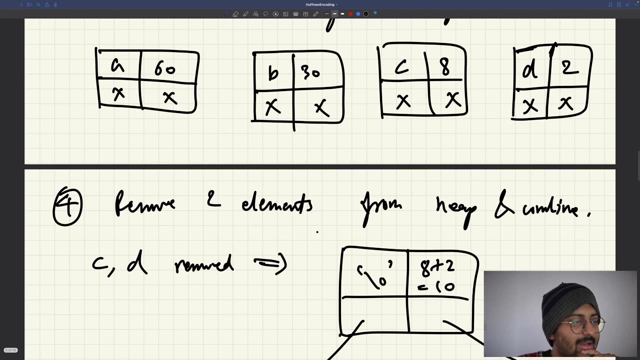 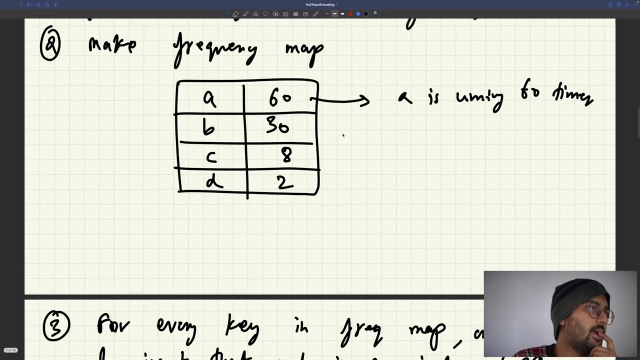 So I'm going to create a min heap- I already created the file for this- And what I'm going to do is I'm going to create a set as well, an entry set. Okay, So what I need to do is every pair in this map over here, as you can see, like A and. 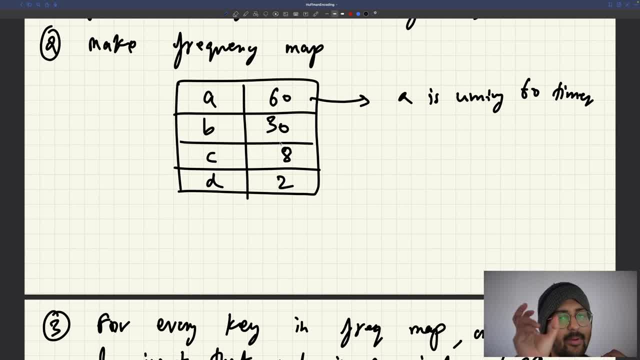 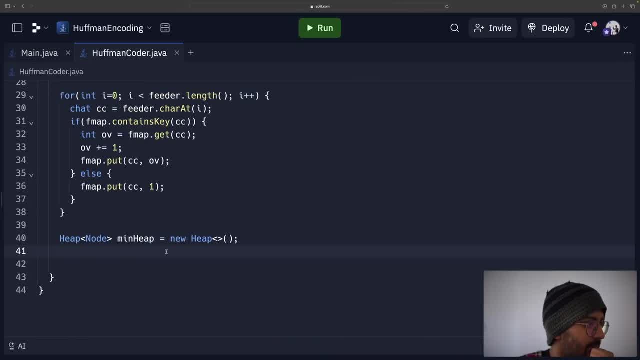 60, B and 30. This is known as a map entry, So map interface dot entry. So I can create it in a set, So I can iterate over this set. For example, I can say: map dot entry, character comma integer. 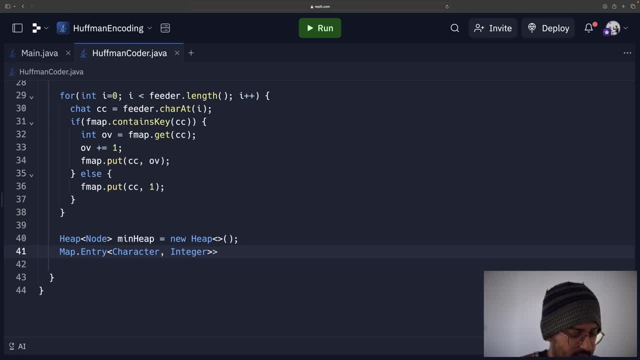 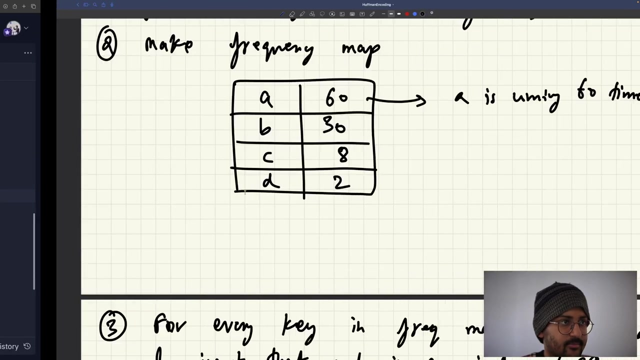 Right, And this is actually I'm going to say set that contains these elements. So entry set from my frequency map I can call entry set. So it will just give me all the sets. Okay, It will give me all these over here. 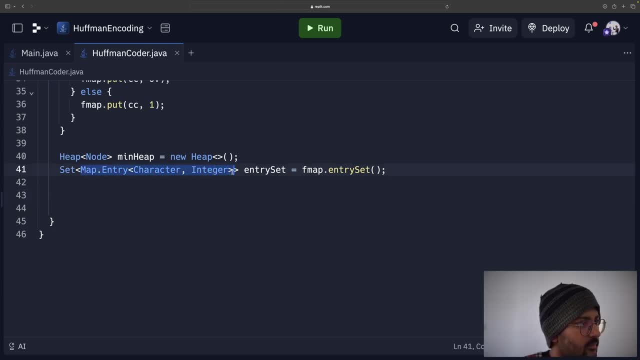 And then I can iterate upon it For every entry in entry set. what do I need to do For every entry individually that I'm getting? I need to create a node Entry dot get key. Okay, I hope this thing is clear. 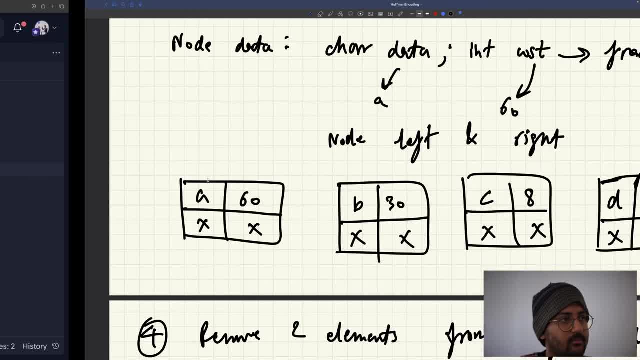 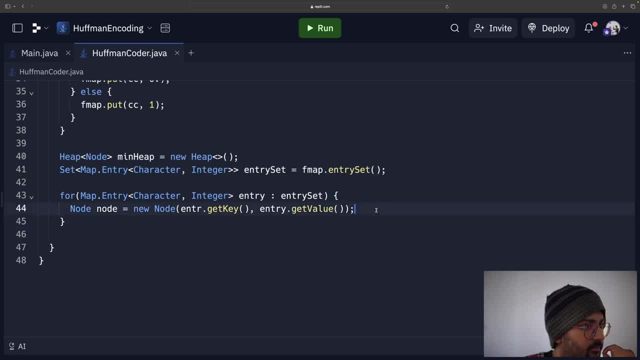 It's just creating a set of all the entries in the map. That's it, This thing. Okay, You can print it as well. It's very simple. After you create the node, you have to insert in min. heap Done. 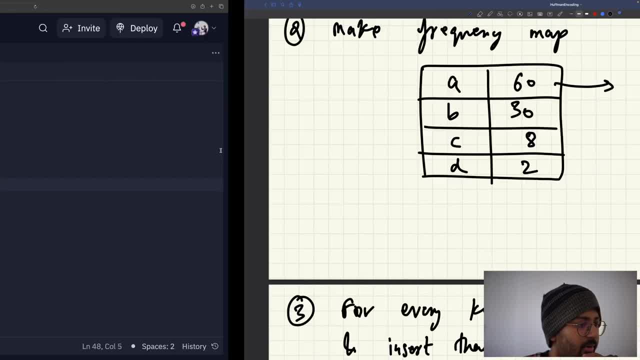 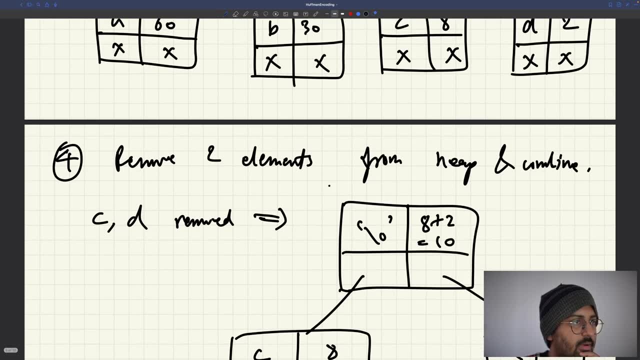 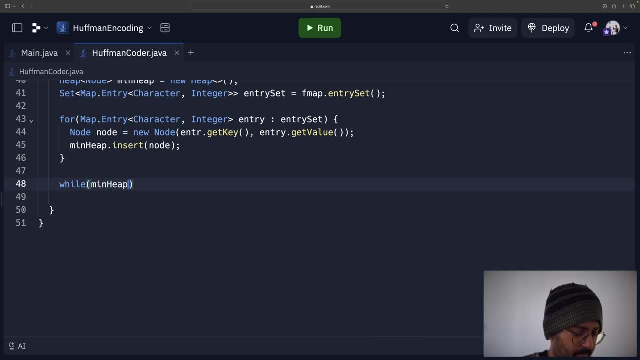 Sounds good. Next step- This I've inserted: Remove two elements from the heap and combine while the heap size remains one. So while min heap dot size is not equal to one, remove two elements. Node first is equal to min heap dot size. 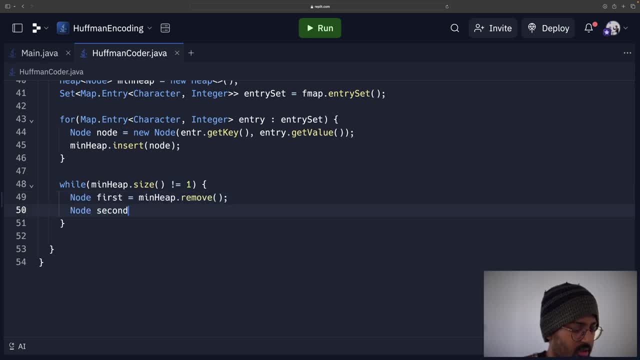 Min heap dot remove. Node second is equal to min heap dot remove. New node will be the one formed by joining them together, Node And name as such. I'll just add here First, and what is the total cost? First dot cost plus second dot cost. 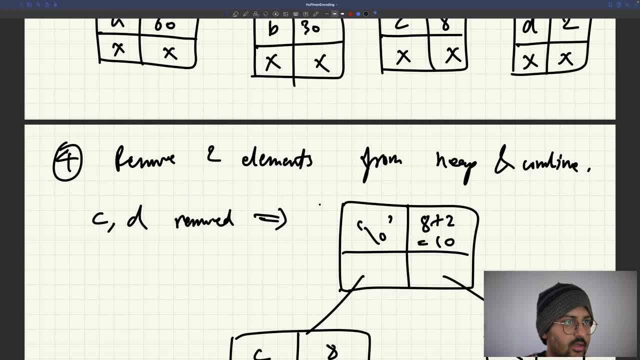 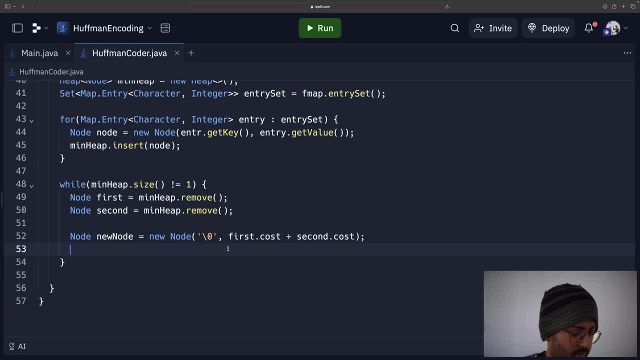 And the new nodes: First dot cost. second dot cost: Left will be equal to the first removed. Right will be equal to the next removed. New node dot left is equal to first removed. New node dot right is equal to second removed. 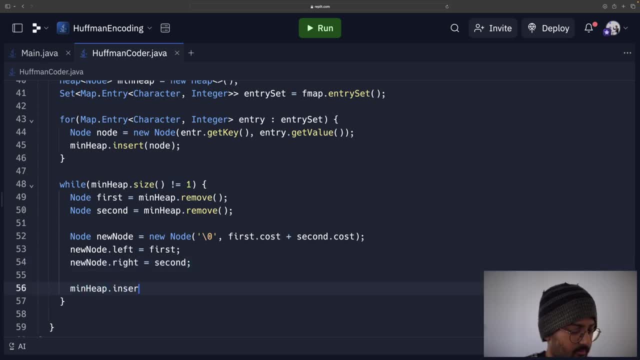 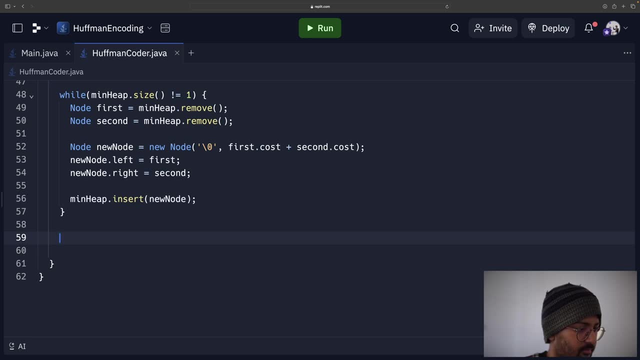 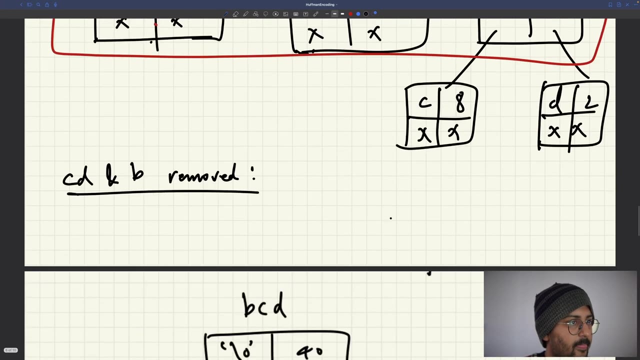 And then I will insert it back in. Okay, After this is done, it will be over. All right, Now we want to create the full tree, which is this one. Let's say, this node is called ft full tree node tree. 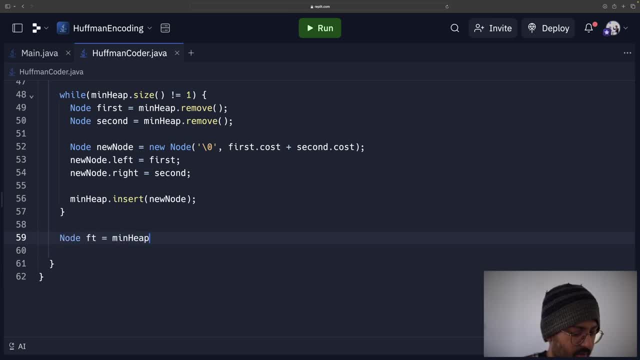 So that will be node. full tree is equal to, I will say, min heap dot remove And I have this node now And using this I have to form encoder and decoder. Okay, So I can say this dot encoder is equal to initially empty. 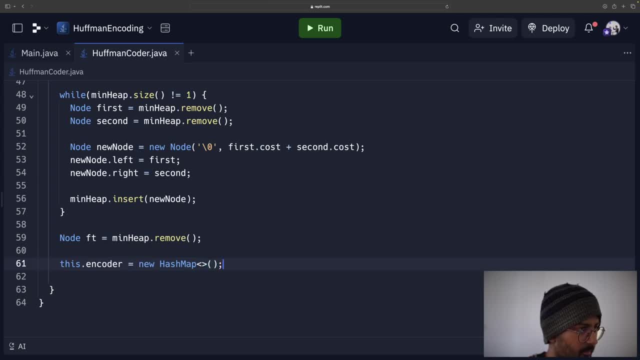 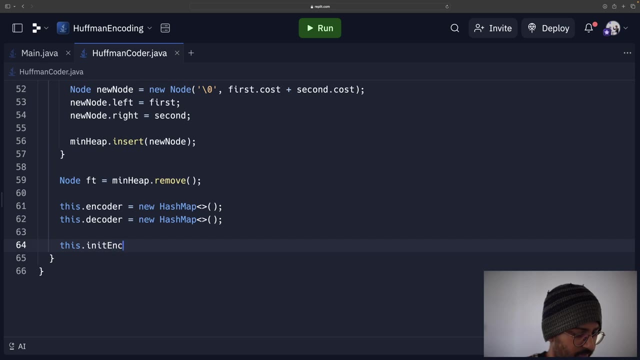 New hash map. Decoder is equal to initially empty New hash map. If I want to fill the encoder and decoder, I can do it in another function: Init. Init- encoder, decoder. I will pass the tree String. initially I'll pass empty. 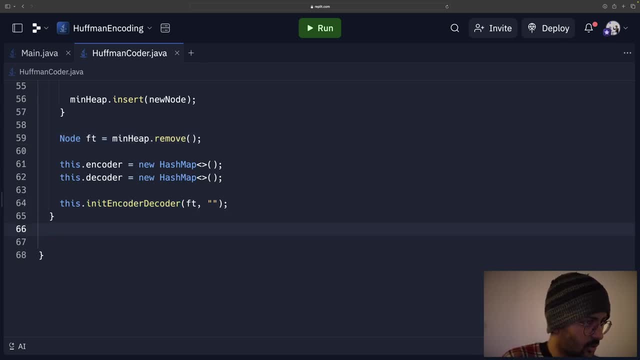 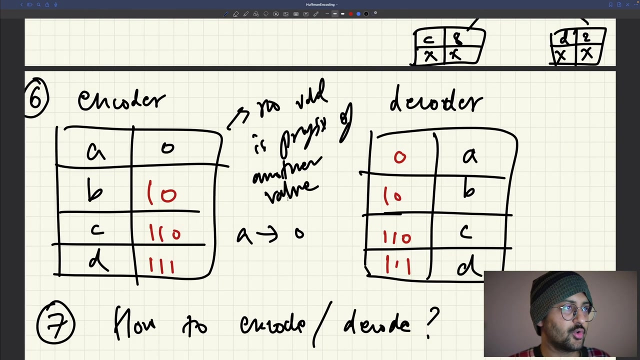 Okay, So here I can create init deco, encoder decoder, And this is going to have a node and string. It's going to contain the output so far That we have, because we're creating encoder decoder, So the output so far That we have. 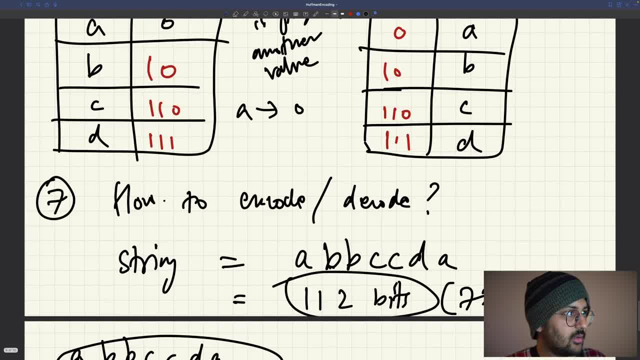 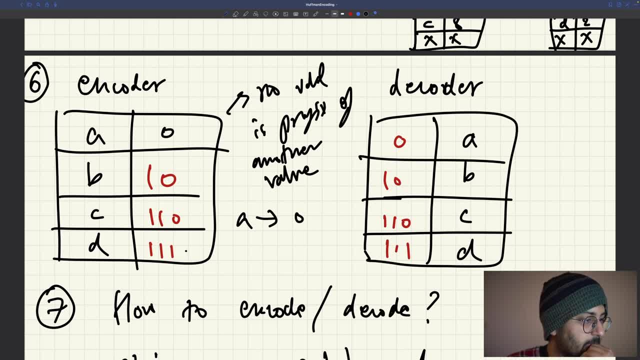 Because we want to calculate right. What is the output so far that we have? Because we are calculating the series 0, 1, 0, 1, 1, 0, 1, 1, 1.. 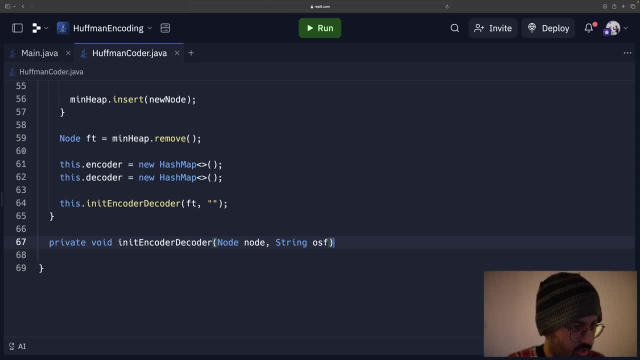 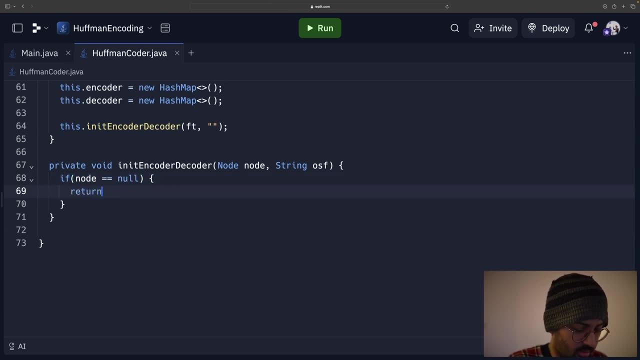 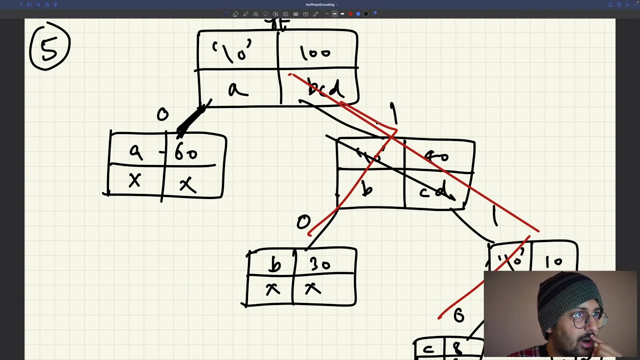 Okay, So output so far? initially it's empty. I can say: if node is equal to equal to null, I will just return. And what I'm going to do is that. what is my output so far? So this is just recursion. I'm going down. 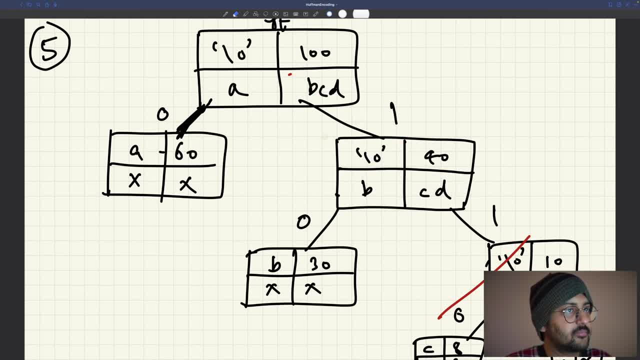 It's just recursion. Okay, So where do I have the path? What is the path, You tell me? Think about it, It's easy. This is the tree given to you. For example, You've done binary search trees, right. 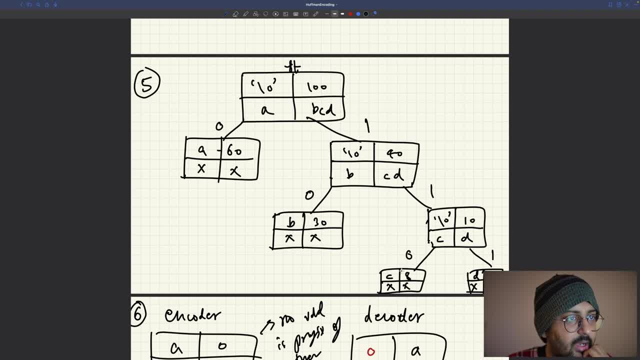 Binary trees. This essentially is like a binary tree format. So this A, This B, that we're getting, This C that we're getting And this D we're getting. Can you see that these are all leaf nodes. So whenever you are at a leaf node, 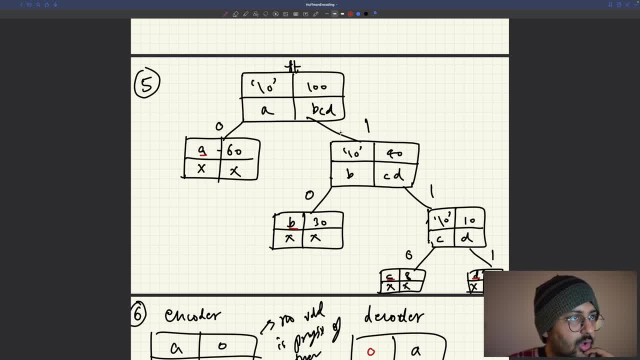 Whatever path so far that you have, Be that 0, 1, 0, 1, 1, 0. Sorry, 1, 1, 1. Or 1, 1, 0. That path will stop when you're at a leaf node. 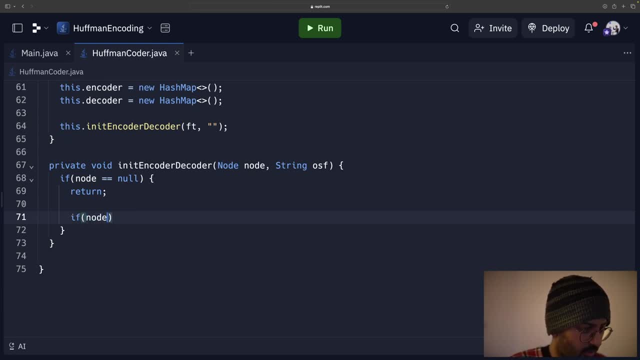 Easy. So if node dot left is equal to equal to null And node dot right is equal to equal to null, It means that I'm at the leaf node. It means that I'm at the leaf node. So I have found one of the characters. 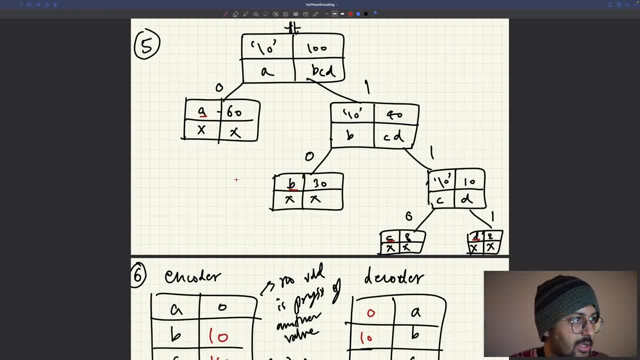 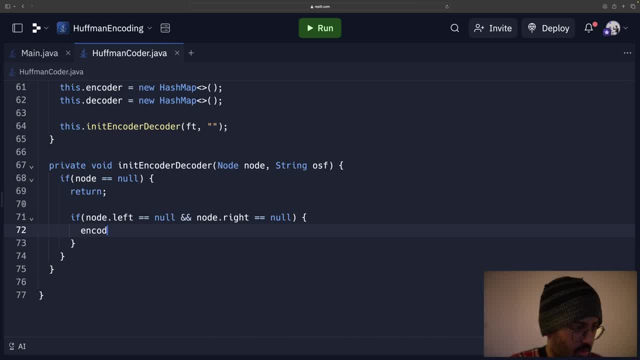 So I will just add that character in my encoder and decoder. So encoder, I will add character, string And then decoder, I will add string and character. Okay, Encoder dot. This dot. encoder dot. put Node dot. data Output. so far This dot decoder. 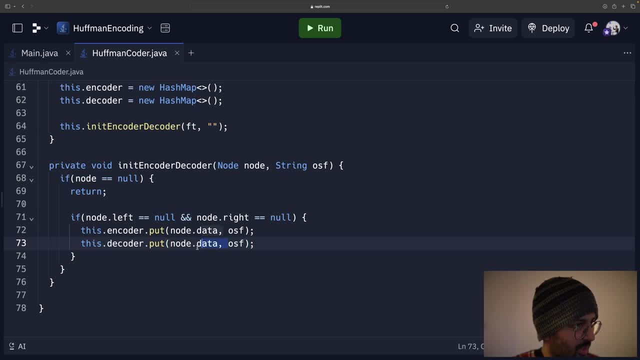 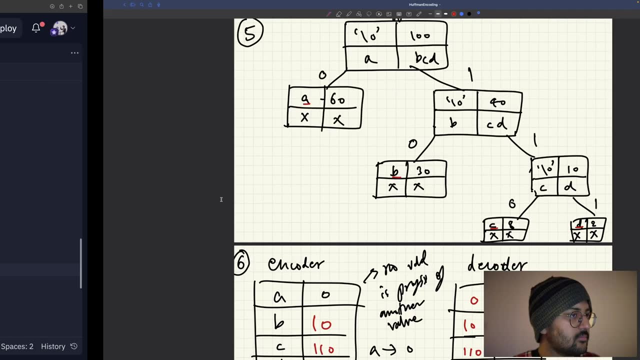 I will put Output so far as keys And then the value will be node dot data. That's it. Otherwise I will just do recursion. I will go left and right. Whenever I go left in the path, I will add 0.. 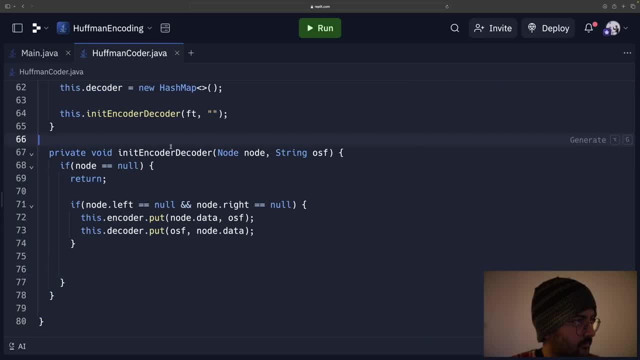 Whenever I go right in the path, I will add 1.. Node dot left Output so far plus. I'm just going to add 0.. Please don't ask me questions about basic recursion. Okay Cool, Because that's not cool. 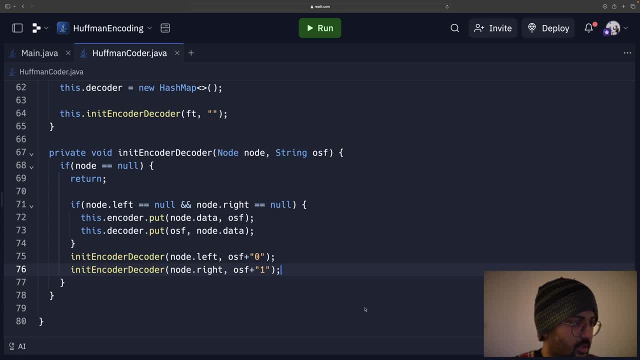 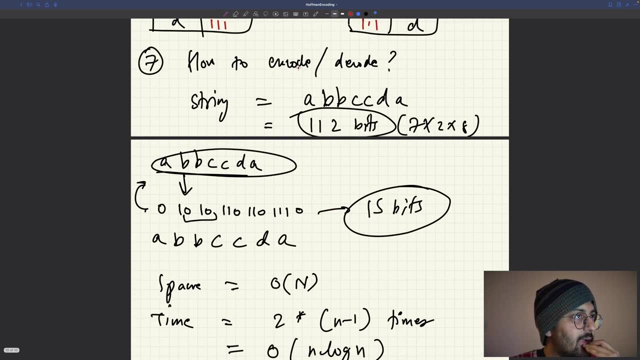 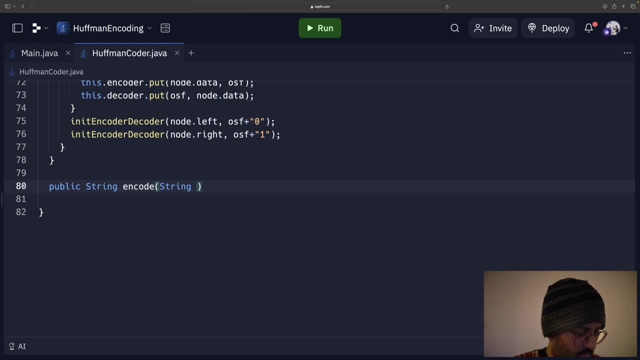 Alright, So that's basically about it. Now, what do we need to do? This table is formed, Now how do we encode and decode? Let's create an encode method and decode method. Let's create an encode method and decode method. We are given a string. 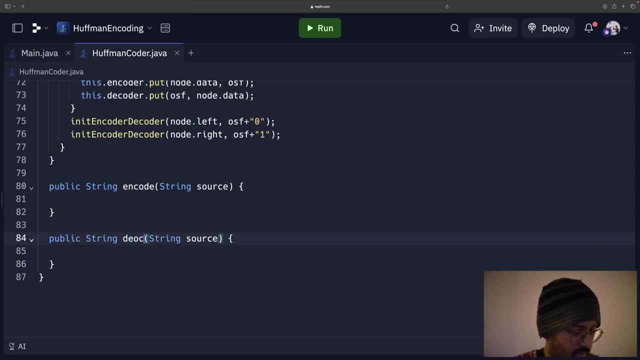 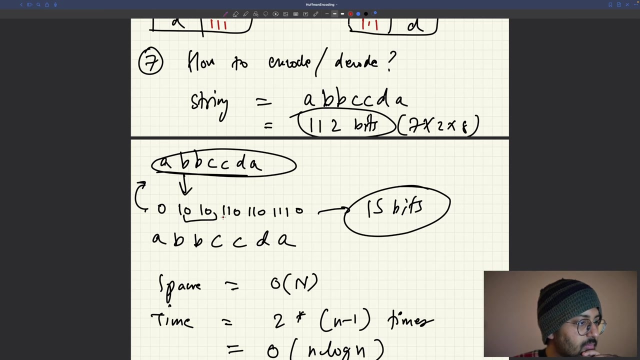 We have to encode it. Similarly, we are given a. This is the message you will give your friend. You are given a, Let's say, coded string and you have to decode it. So how do you encode a string? How do you create a string into? 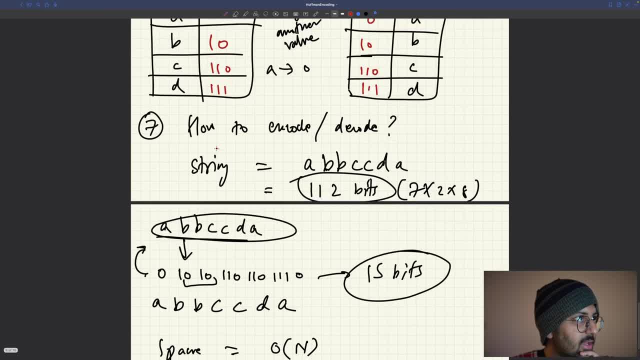 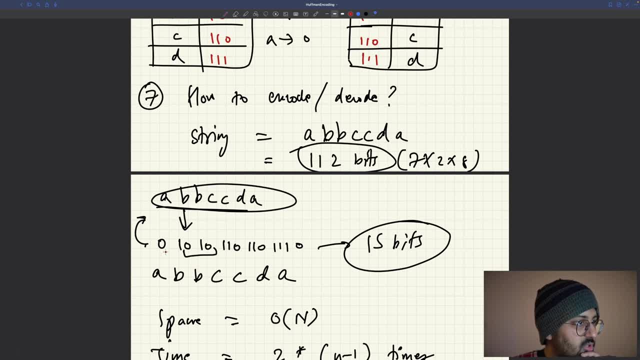 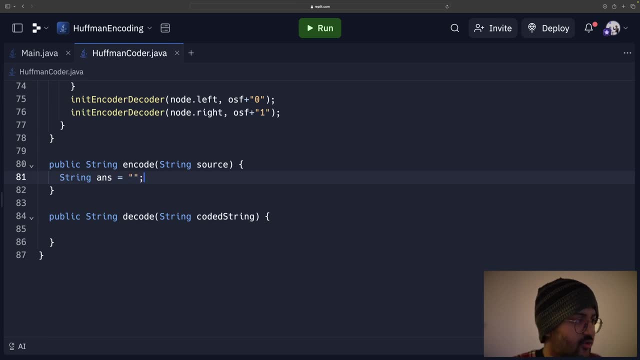 So you take a And you will just take the value, And you will just take the value of a, Which is 0.. And I will just put it in my String. Answer is equal to. You can use string builder, But I am lazy. 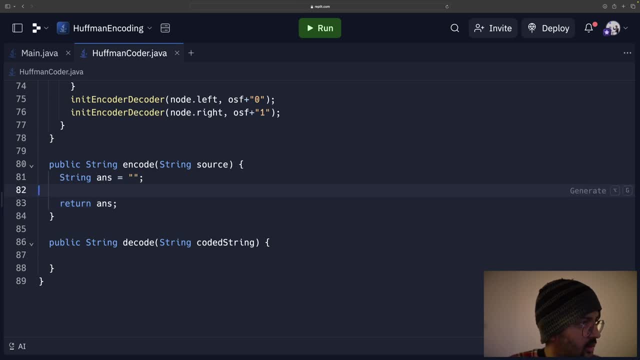 So I will just Do it like this, But please use string builder. Okay, I have taught you string builder before, So Traverse every character. Answer plus Encoder dot. get the character. That's it. How will you decode? You are given this string like this: 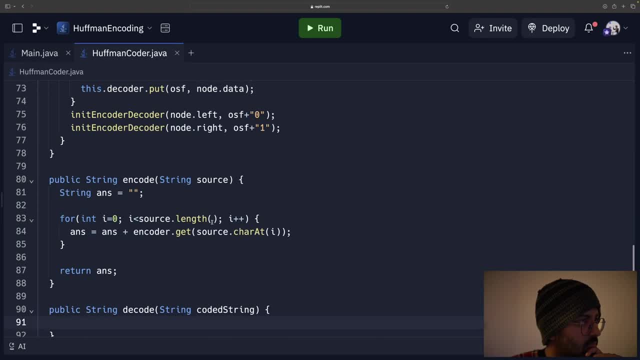 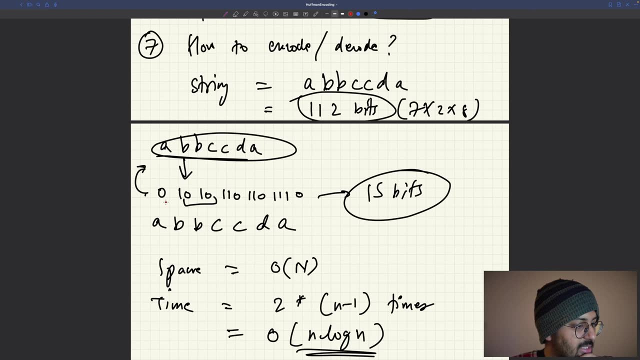 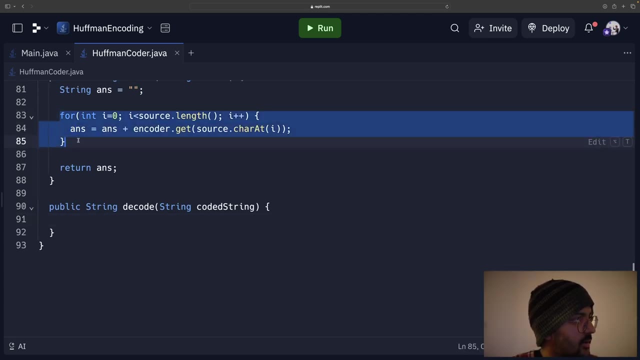 Okay, You are given 0. So you will start using 0.. You will first of all go one by one. Okay, So that's fine, Coded string dot length. I will go one by one. But what will I do? 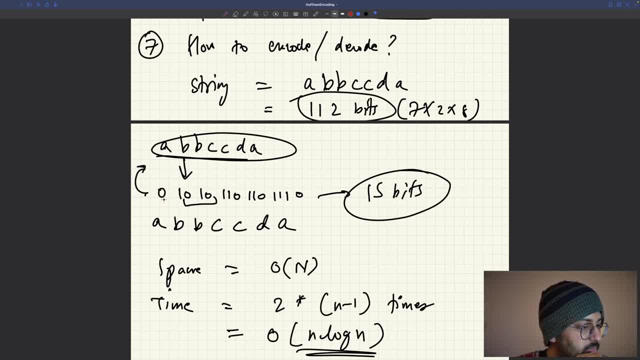 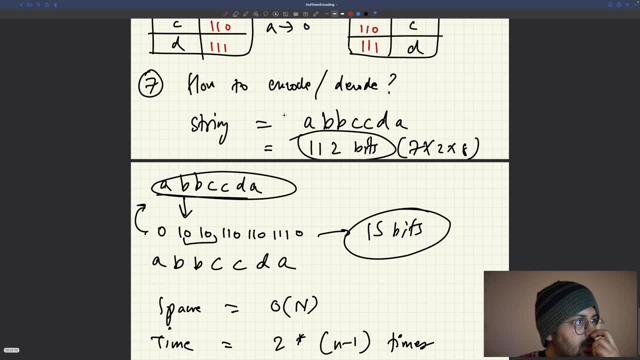 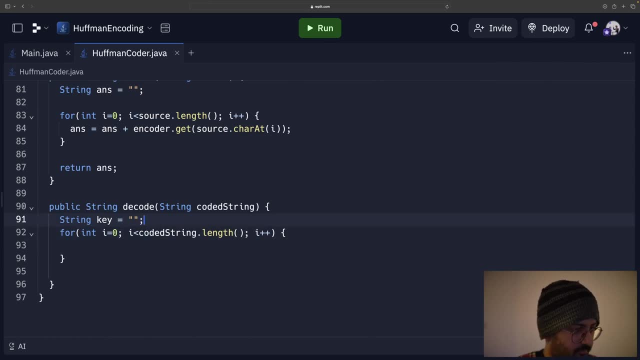 I am at index 0.. I have to find my key 010110 or 111.. So I will take a key. Key is equal to initially empty. I will say: key is equal to key Plus. Coded string: dot. 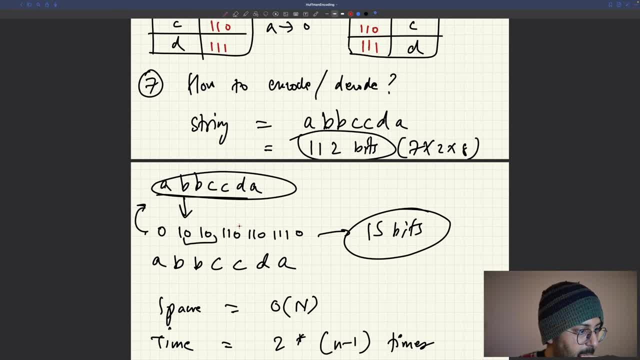 Carrot I. So I have my key now As I move forward. Okay, If So, I will be like: Okay, Let's say I am here At 1.. Does My hash map, This decoder, contain 1.. 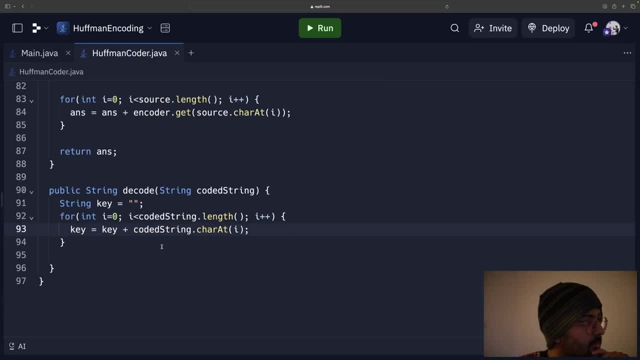 No, it doesn't. Then keep moving forward. Right? If it contains key, Then I will just Add it. in my answer. I will say: answer Is equal to answer, plus Decoder Dot, Get The key. This will give me the character. 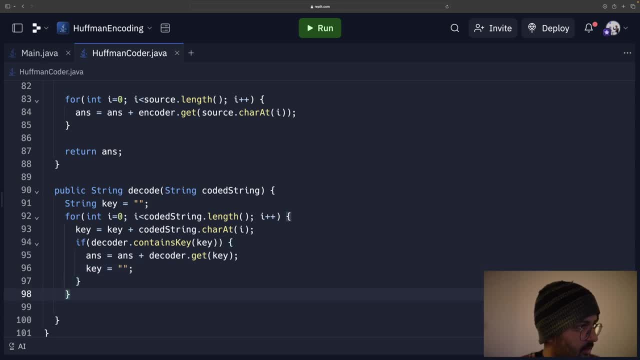 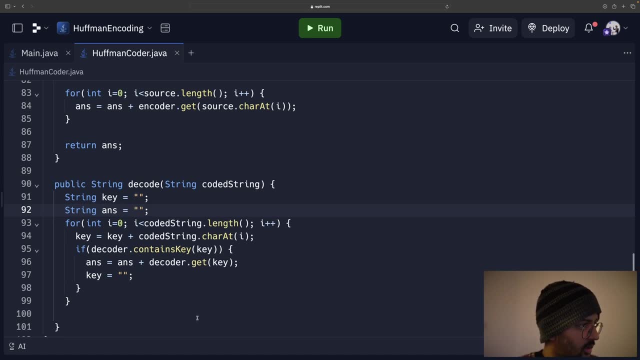 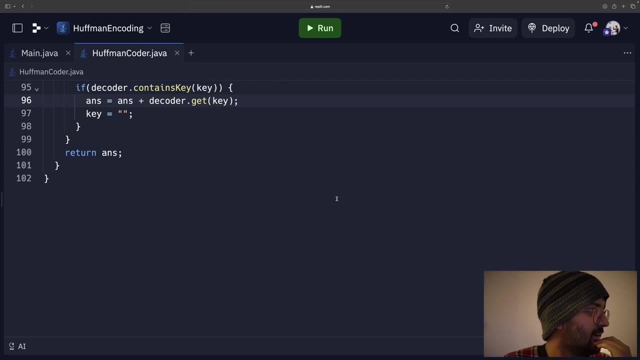 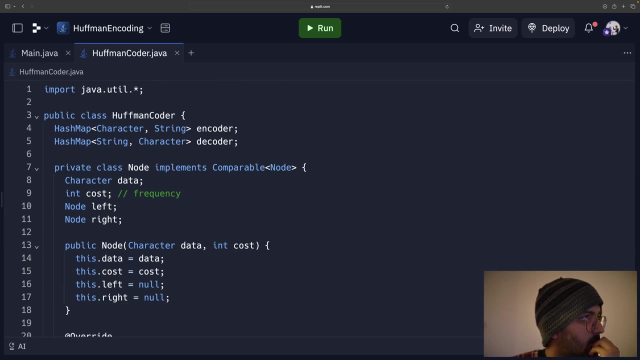 And now key will be reset to again empty And I need a string answer also. In the end, just Return the answer. That's it Done. Huffman coding, That was it. Cuckoo Sounds good. Okay, Easy what I did. 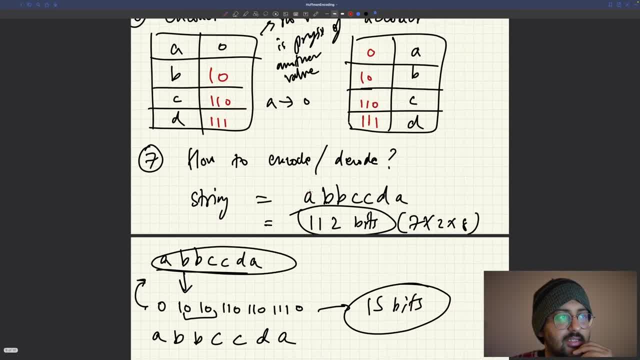 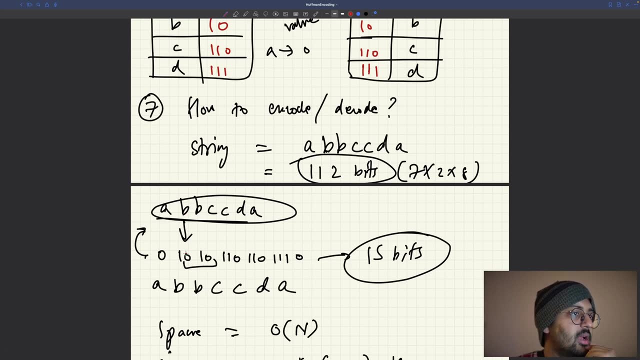 Encoding and decoding. I was just taking. Encoding was easy. Just take A And whatever the value of A is, Put that in a string. Similarly for B. Whatever the value of B is, Put that in a string. Now I know it is being stored in string. 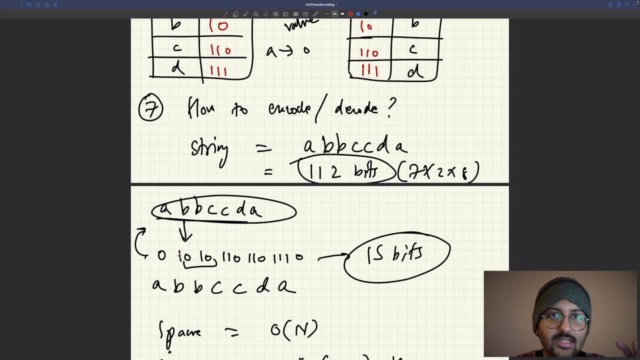 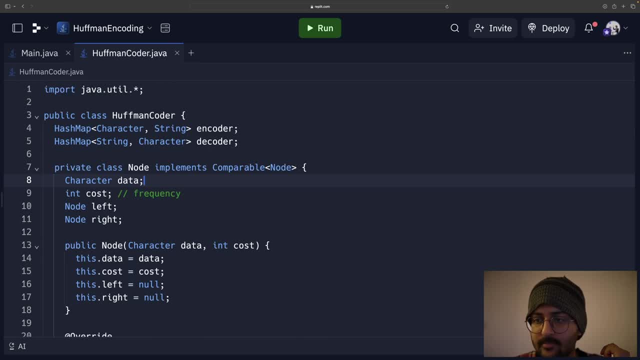 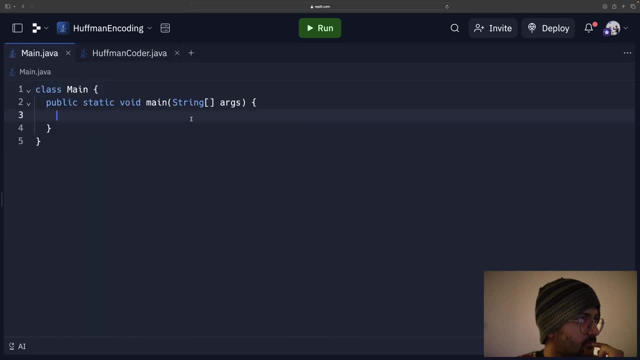 But I just wanted to show you the mechanism. You can put it in bits as well, You can do whatever you want, But this is. I wanted to show you the mechanism. Let's run this, Okay, Throws- exception String. I'm going to say: 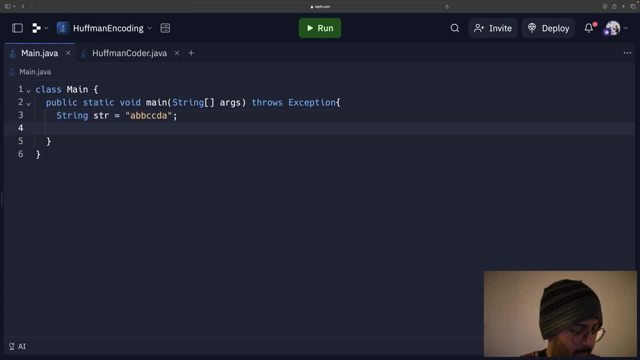 A, B, B, C, C, D A. Huffman Encoder. New Encoder String Say: string Coded string is equal to Window encode. The string Decoded string is equal to Decode Coded string. 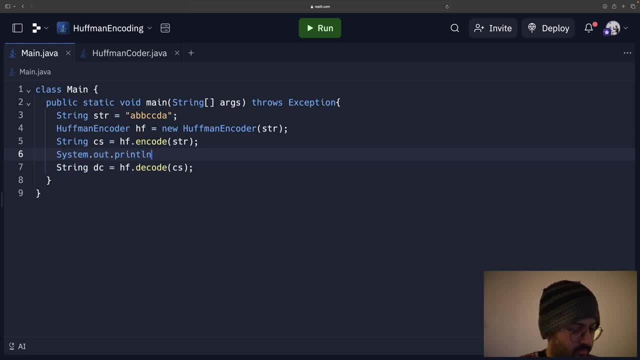 Let's print it as well. Coded string. Decoded string. Okay, So what? I would recommend it you can, You know, In order to make the best one. It's set Can be used, So it's Like an. 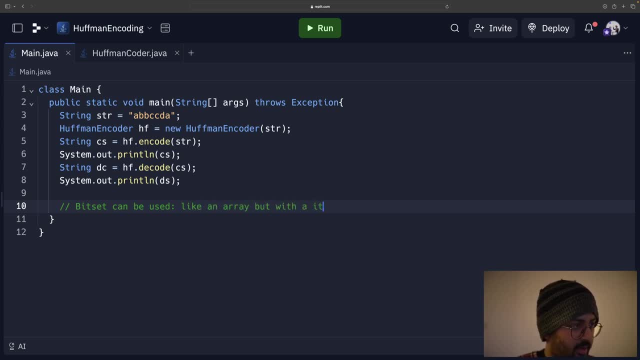 Array, But With A bit At Each Index. Okay, That is what I would recommend. Try to run this. Okay, Just pick some Typos And Commas And Stuff. Let's run this. 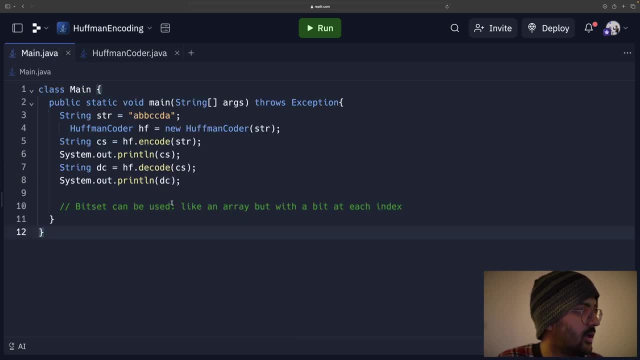 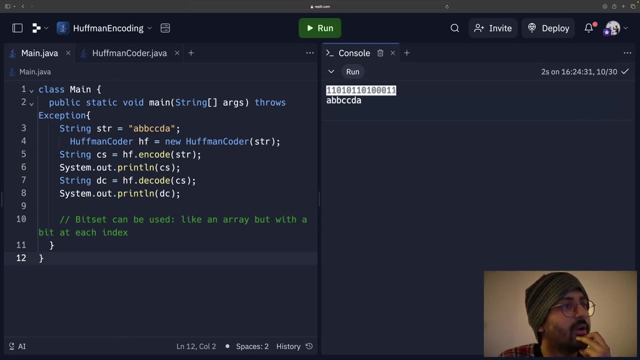 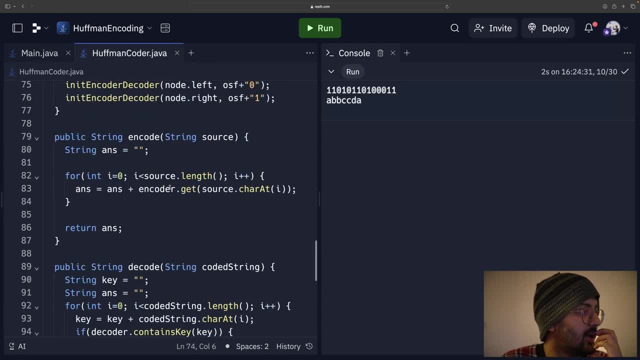 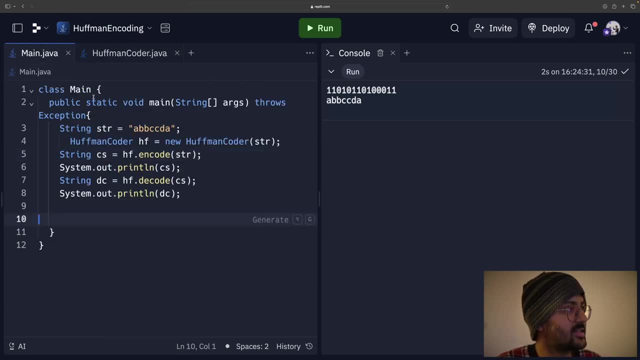 Easy. I know I'm storing it As strings Right now, Don't worry, I know, I know that here I'm storing it, as You know, Here as a string, But you can, I'd say, Bit set.